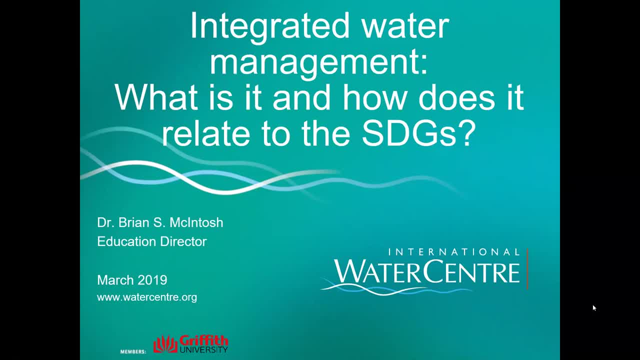 suitable approach for delivering the SDGs. Brian McIntosh, I'm the education director here at the International Water Center, or IWC as we call ourselves. There will be an opportunity for some questions at the end And on the last slide that I'll 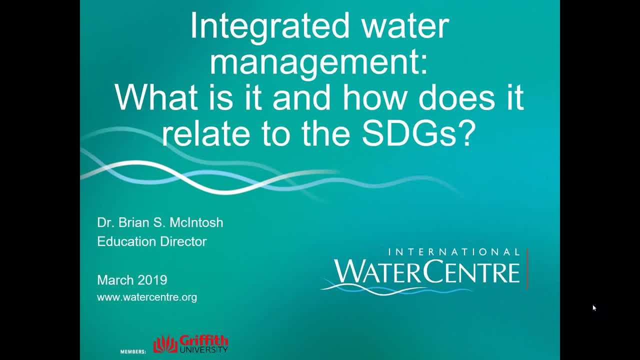 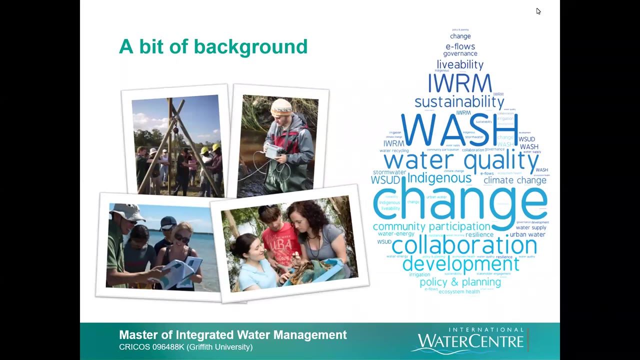 show. I'll also have some contact details should you wish to follow up by email or Skype or even by phone. Just a little bit of background. Let me get the slide forward. Here we go. I'll just briefly say something about the IWC. So we're a capacity building organization based in Brisbane which is 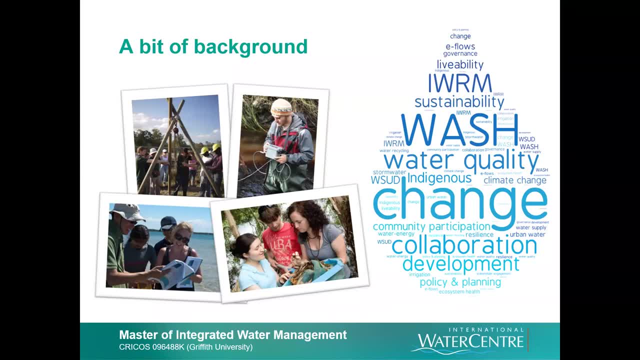 located about the middle of the east coast of Australia in the state of Queensland. Queensland is famous for a lot of things. We've just had a major drought and a major flood, But we are at the place where the Great Barrier Reef exists, just off the coast, for sort of 1,500 kilometers, 2,000 kilometers of the coast. So we've got a lot of. 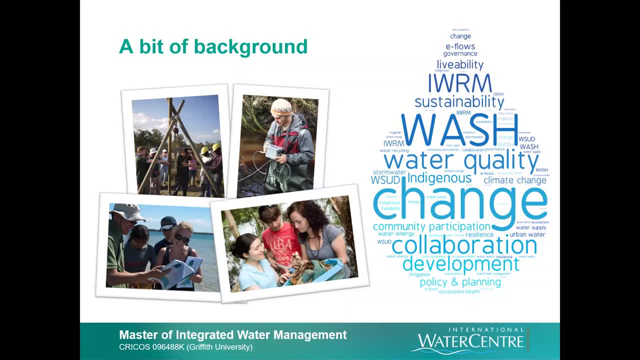 things in place. So we're a capacity building organization based in Brisbane which is located about the middle of the east coast of Queensland, which is a big, big, long state. One of the main activities of the IWC is delivering a professionally 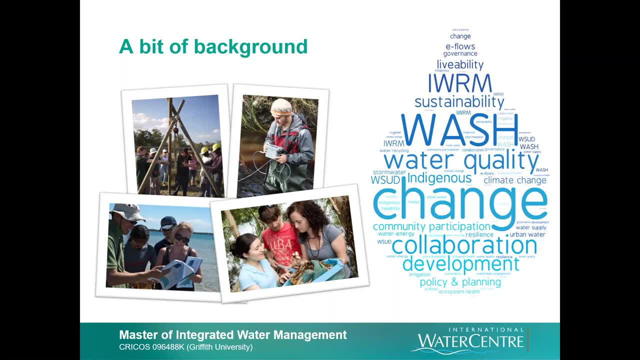 oriented Master of Integrated Water Management And that's a program that seeks to build the kinds of practical knowledge, skills and capabilities in individuals that we view as as being necessary to respond to global water and sustainable development challenges. We've had the program running. We've now got the 11th cohort. We've had it running for 11. years with the explicit purpose of building a community-based water system, And the most important thing for us is that we've we've had the program running. We've now got the 11th cohort. We've had it running for 11 years with the explicit purpose of building a community. 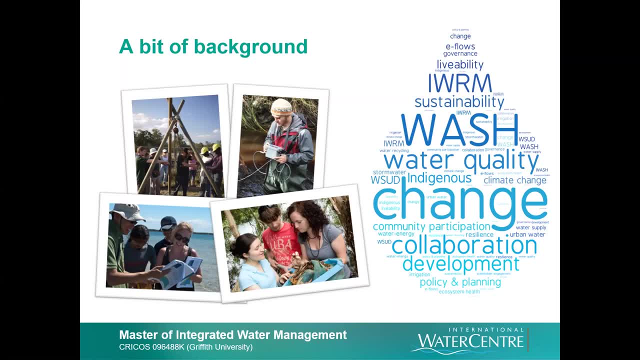 have engaged effective change agents really working across the world to transform the way that we think about and act to manage water, and we've got this community now spread across 86 different countries. That's just a little bit of context about us. We do training and online training projects and a bunch. 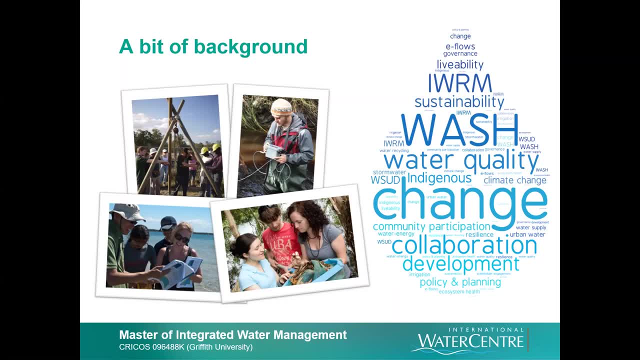 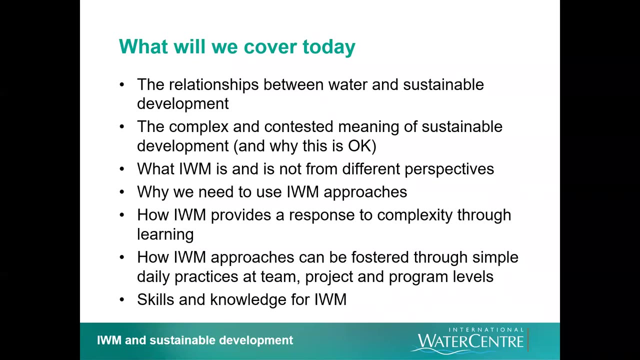 of other things, but all focused really on capacity building and building capacity for the implementation of integrated water management For this webinar. I suppose what we want overall for you from this webinar is to have been exposed to our interpretation- and I use the word interpretation quite deliberately- our interpretation of integrated water. 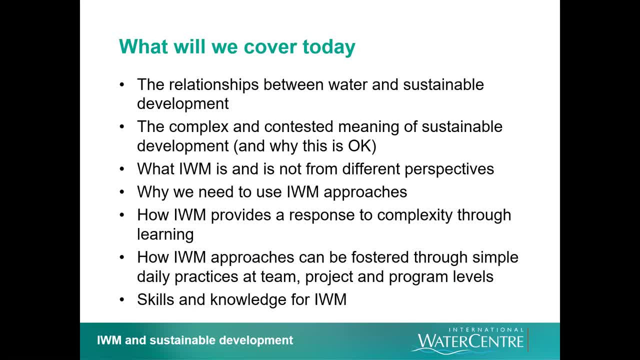 management What it is, why it's significant as an approach for delivering the SDGs. The bullet points on the slide in front of you show them the main areas that we're going to cover in more detail today. So we're going to be looking, I suppose, at the relationships between water and 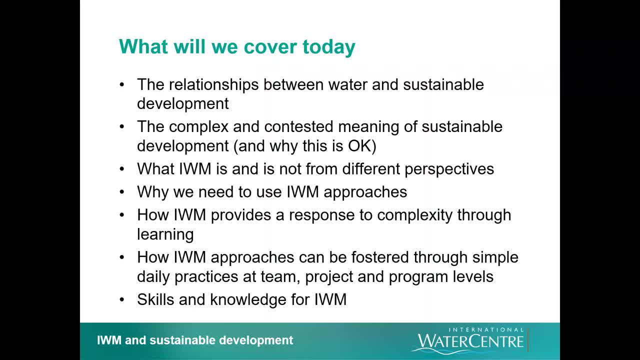 sustainable development. We'll be looking at the complex and contested meaning of sustainable development and why that's okay. We'll be covering what IWM is and is not, from different perspectives, creating the case for why we need to use IWM approaches, detailing, I suppose, how IWM provides a. 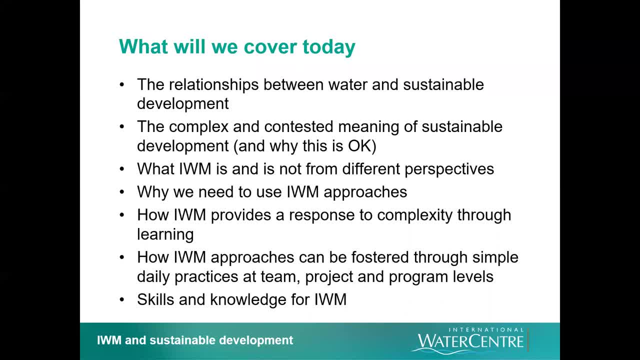 response to complexity through learning and remembering that complexity is a fundamental, I suppose, characteristic of sustainable development, And how we'll also be covering how IWM approaches can be fostered through simple daily practices at team, project and program levels, as well as through the 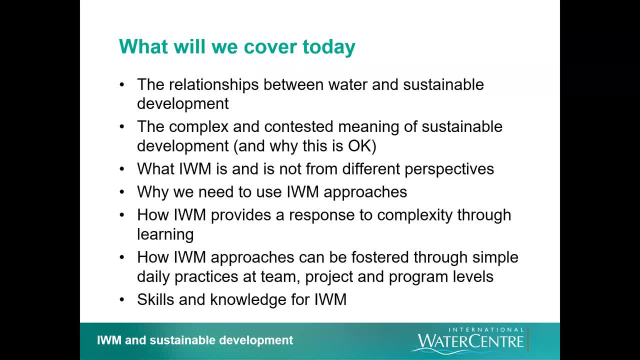 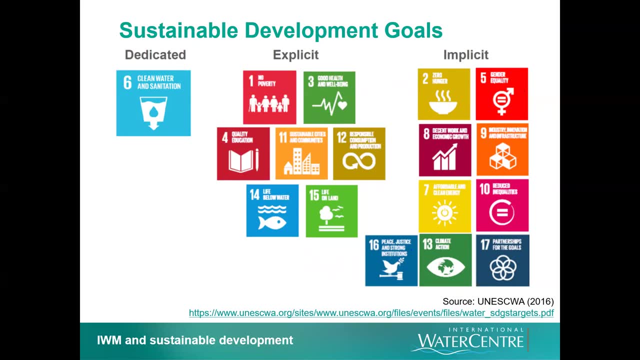 development of particular kinds of skills and knowledge profiles in professionals and in organizations. To get started, what I'd like to do is turn our attention to, I suppose, to sustainable development and water. The United Nations Economic and Social Commission for Western Asia, UNESCOA. there's a link on the screen in front of you. they provide 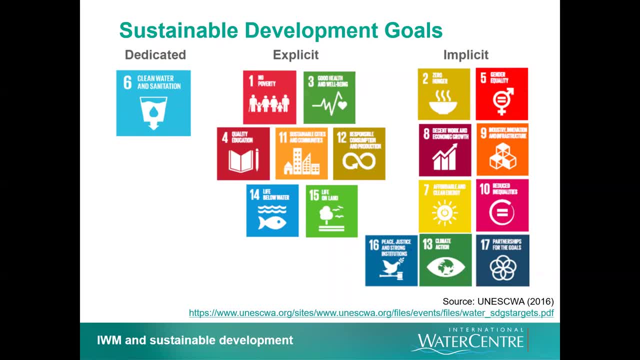 what I think is a great way of seeing the relationships between water and sustainable development by categorizing the SDGs. The SDGs are perhaps currently the most famous operational definition of sustainable development. Certainly, I think what we find is it's known in professional circles, maybe not so well known in the general. 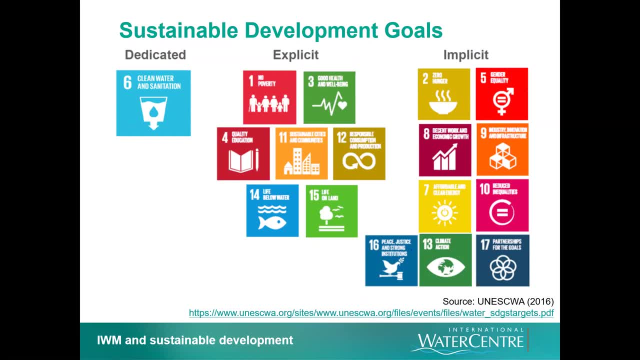 general public. but the SDGs are not the only definition of sustainable development and it's worth making sure that that's maybe not at the front of your mind, but somewhere fairly close to the front of your mind. UNESCO's diagram that's on the screen in front of us. 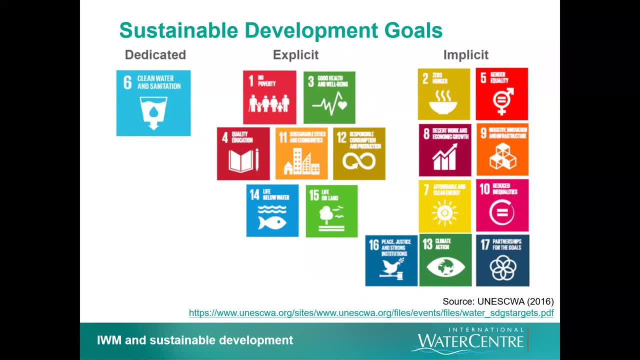 it shows how water is really unsurprisingly central to the achievement of sustainable development. so there's a dedicated SDG, SDG6- that I'm sure you're all probably familiar with. But UNESCO's diagram also shows how water is explicitly a part of achieving a further 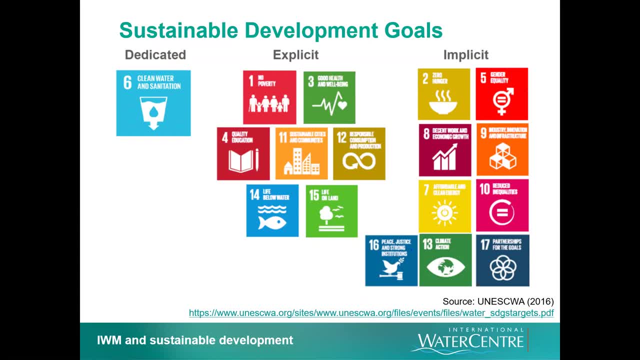 7 SDGs and that it's directly or implicitly a part of achieving a further 9 SDGs, and it means really that water is directly, explicitly or implicitly a part of achieving all 17 SDGs. This really, I think, speaks to why people get involved in water and water management. 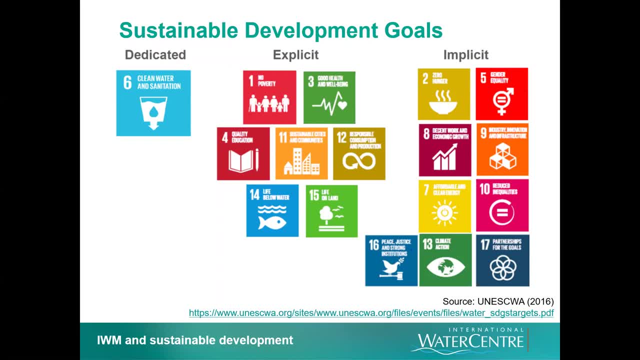 Water is essential to achieving sustainable development. Almost everything, either directly or indirectly, depends on water. It's a meeting ground. it's a meeting ground for people who are interested in tackling some of the most complex and interconnected challenges that face our people. 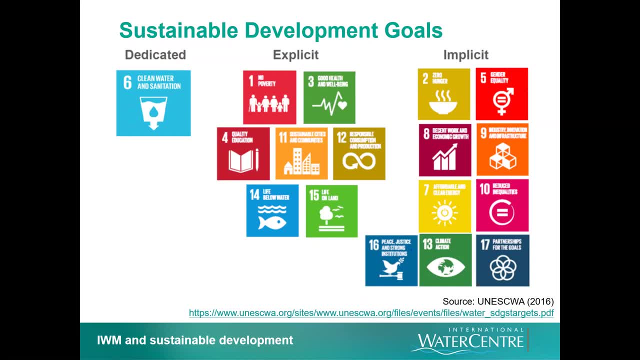 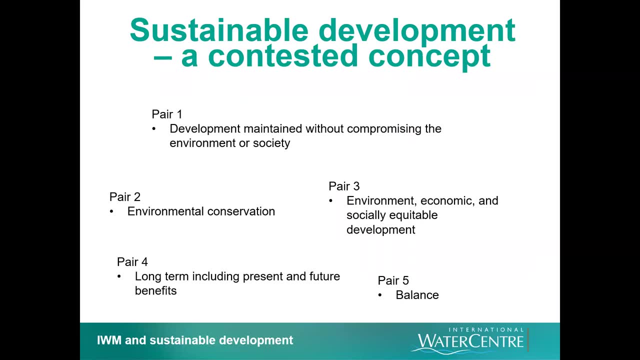 Our countries and, globally, the world. If we take the SDGs as a definition of sustainable development- and that's not a crazy thing to do, but bear in mind, they're not the only definition of sustainable development- you might say great. so we know what sustainable development is and we know what role water 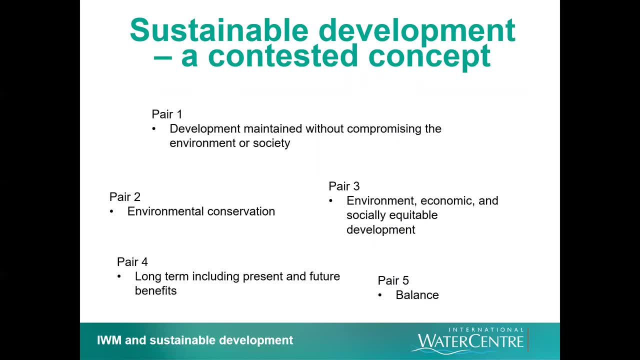 plays in delivering it, and I suppose well sort of Sustainable development is ultimately the aim of integrated water management. It's easy to forget that integrated water management is a means. It's not an end in itself. When people find they have a great approach or a great tool, they tend to go around looking. 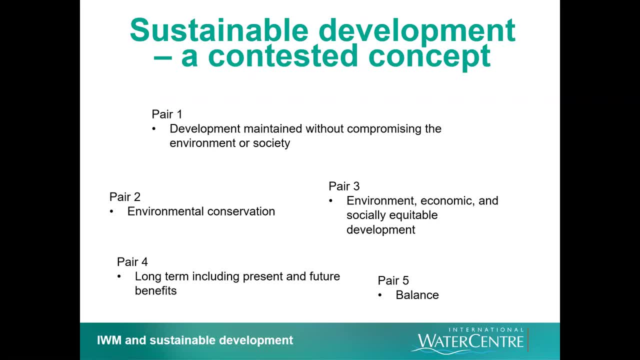 for ways to apply that approach and tool and sort of forget that the approach or tool isn't really the end objective, It's whatever the approach or tool enables you to do. So IWM is an approach or a tool, a means to achieve sustainable development, but what? 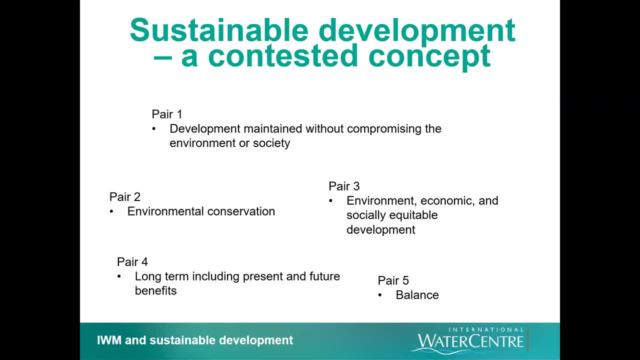 sustainable development is and means is contested, regardless of how widely accepted the SDGs are. Take what you see in front of you. This was the outputs of a very brief exercise with a small set of our master's program participants. I'd ask them to form pairs and then to write down the most important three meanings of. 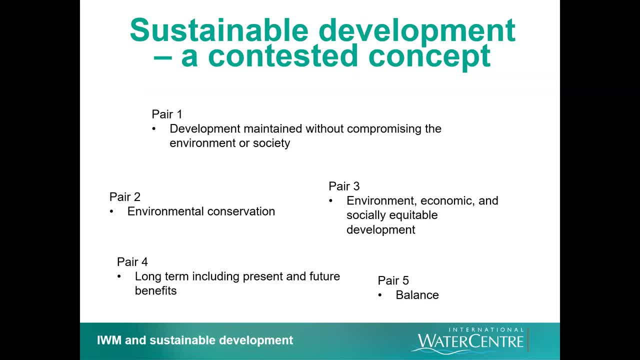 sustainable development. The first two, the first most important meanings they identified in their pairs, are shown on the screen, and no two of them are the same. All of them use terms which themselves require further definition and which are open to further debate and differences of view, such as equitable development, balance, environment benefits. 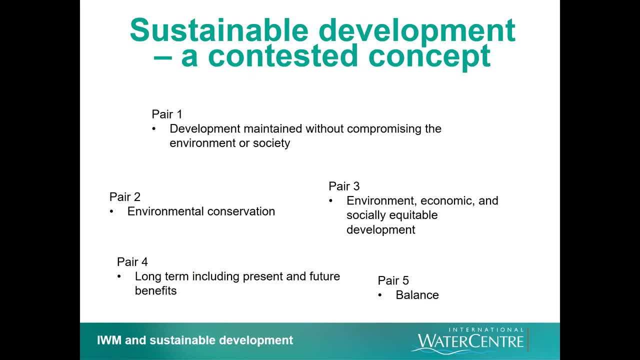 And all of this is okay. Sustainable development is an example of what sociologists sometimes call a boundary object. That is, it's a concept which offers sufficient precision and meaning for different people to engage in discussion about it and, through that discussion, to generate further meanings. 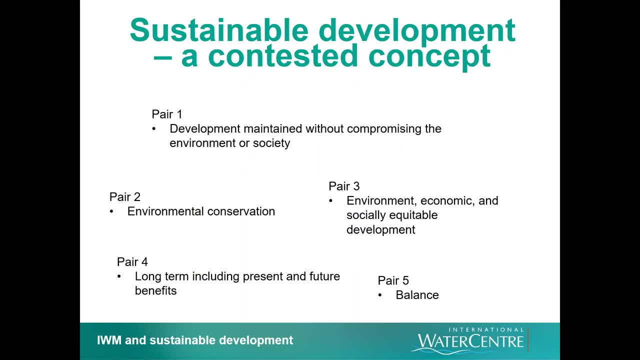 and hopefully, agreements on action. But if sustainable development is a contested concept, then what does that mean for the application of an approach or a tool? What does it mean for IWM, given that IWM can be seen, or should probably be seen, as 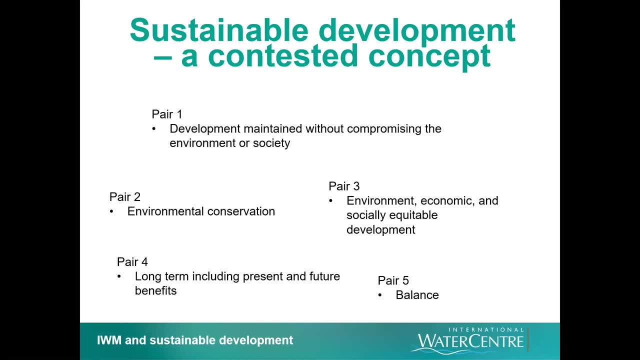 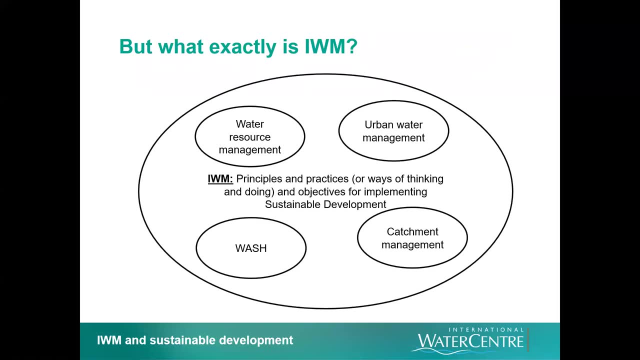 a tool or an approach to implement sustainable development? To answer that question, what I'll do is I'll start by outlining a framework for IWM which positions IWM as a set of principles or practices or ways of thinking and doing and a set of management objectives for the purpose of achieving or implementing sustainable 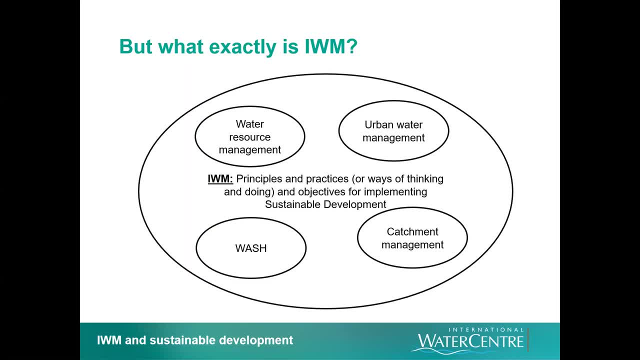 development, Or at least the water. That's a pretty common way of thinking, But, as we've seen on a couple of slides ago, there's not much of sustainable development that is not in some way related to or dependent upon water. Thinking about IWM in this way enables us to then think about IWM as a general approach. 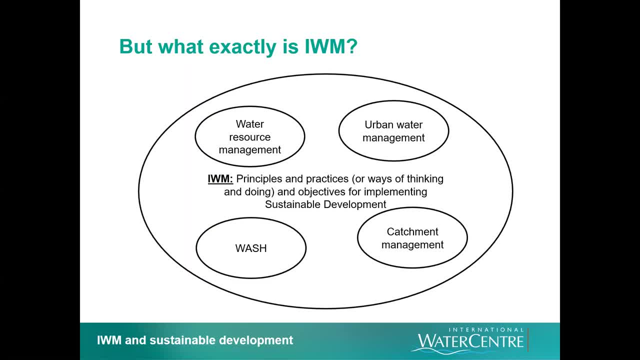 which can then be applied to different areas of water management, areas that correspond to the practical work that that's undertaken every day across the world's water sectors. For example, IWM applies to water resource management. is IWRM- Integrated Water Resource Management- Applied to? 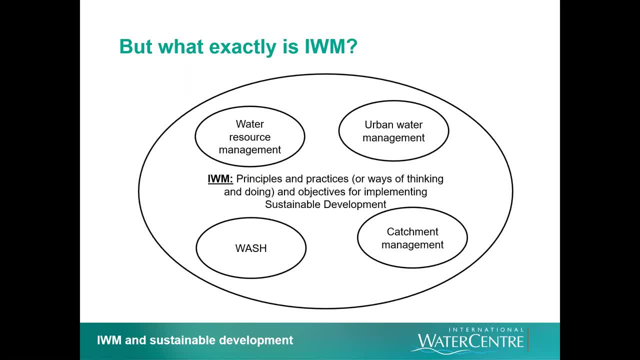 Urban Water Management is IUWM- Integrated Urban Water Management- And you know it's important not to get too hung up on the labels. but a question that we often get is: why is it IWM? Why is it not IWRM? 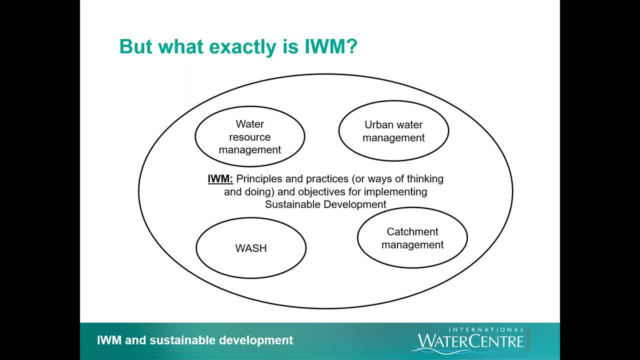 And for us it's the same thing. It's a set of principles, but which have been applied to just specific application area: water resource management. Okay, so if IWRM is a set of general principles and practices, what are these general principles and practices? 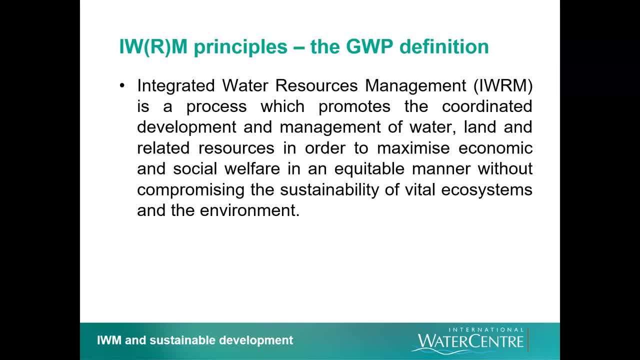 We can find, I suppose, lots of different articulations of these general principles and practices in different places, according to application area. For example, if we look at the definitions of IWRM, like the ones provided by the Global Water Partnership, or GWP. 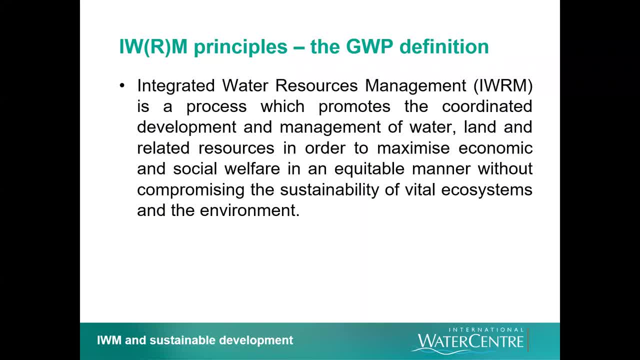 we'll find we're putting principles like the ones in front of you. So coordinated development of water, land and related resources. This implies that IWM or IWRM is concerned with somehow coordinating policy planning and management across sectors and resources. Maximize economic and social welfare. 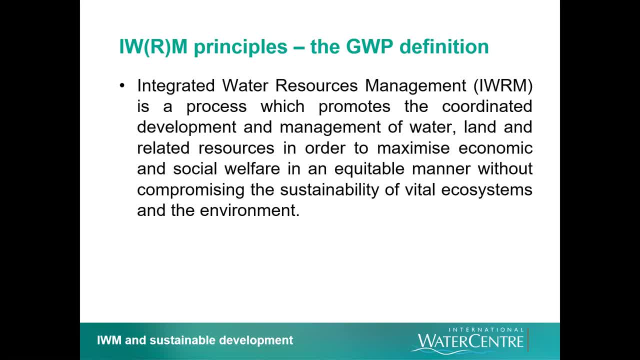 without compromising vital ecosystems. This implies that IWM or IWRM is concerned with ensuring that water is managed in a way that respects the triple bottom line of sustainable development, But in an equitable manner. this implies that IWM or IWRM has a focus on fairness and justice. 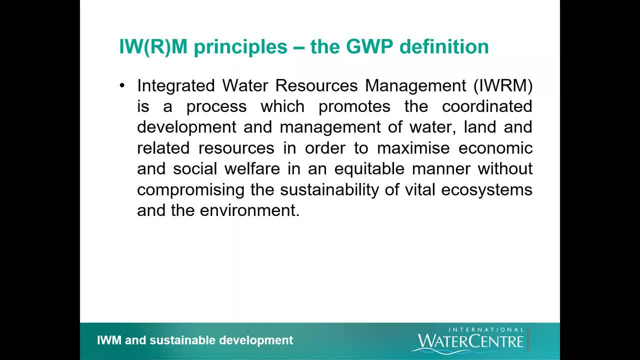 in some way, which I guess are some of the foundations of social sustainability. One way to think about principles such as the ones that you see encapsulated in that GWP statement in front of you is that they are compasses that point towards sustainable development. 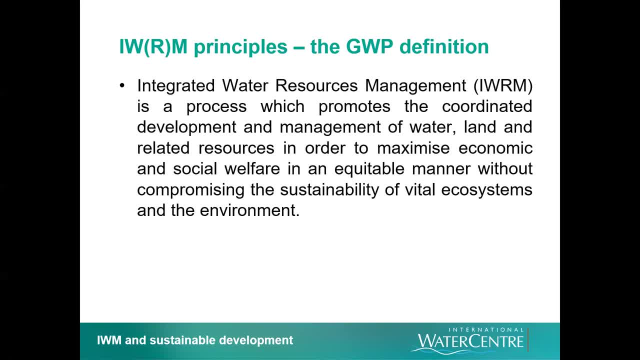 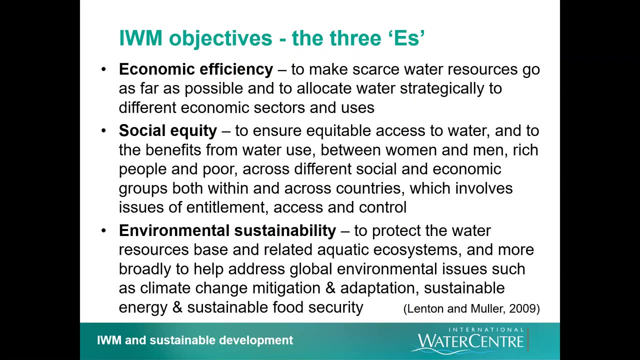 Another way to think about them is that they encourage us to focus holistically at the whole system level, rather than in terms of parts treated separately. We can also find examples of general IWM objectives, such as the three E's of economic efficiency, social equity. 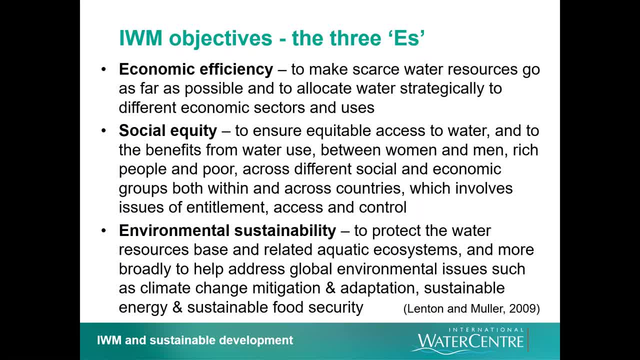 and environmental sustainability that we must somehow try to balance in some way together. The act of balancing these objectives together is what makes water management that attempts to do so integrated in some way. That's one view of what makes the integrated in IWM or IWRM. 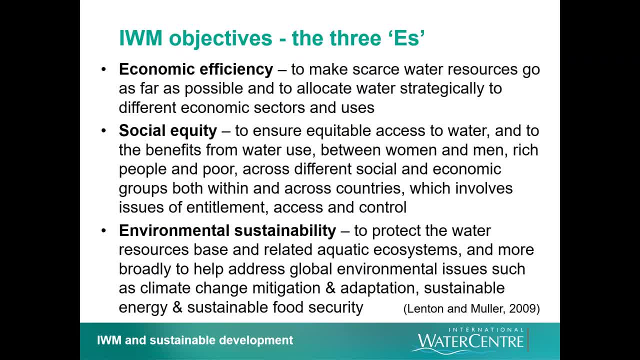 And again, this articulation of objectives points us both towards sustainability, but they also offer a bit like the previous GWP definition: they offer us a framework and they push us towards thinking and acting systemically to achieve multiple objectives. They push us away. 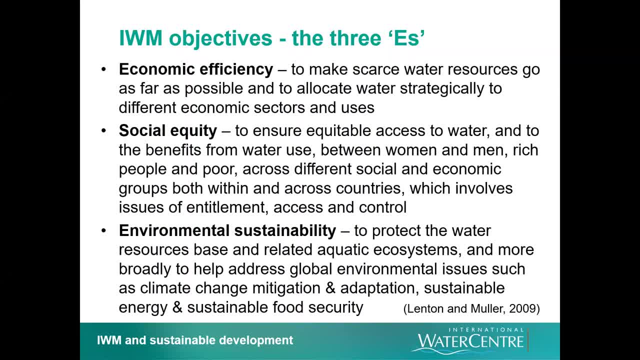 from thinking of the world and managing the world in separate boxes and push us towards managing water resources or other whatever aspect of water we're managing, in a much more systemic way. So that's fine and fair enough. You know we've got these sort of systemic 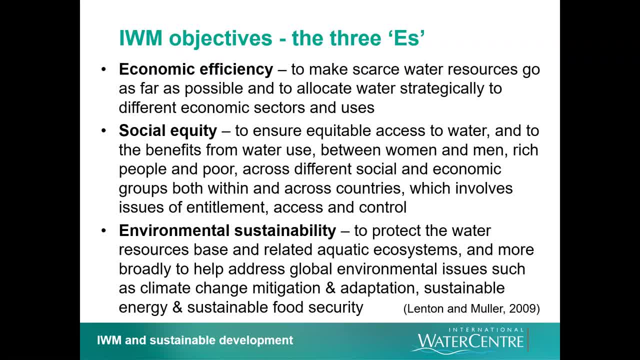 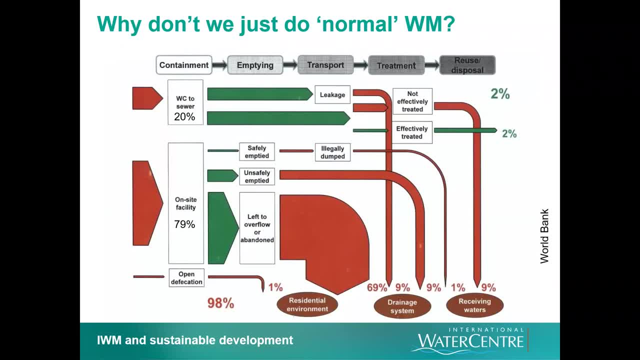 holistic, sustainability oriented principles and even management objectives. It's good to ask, well, why should we utilise these kinds of principles and objectives to guide our work in water management? Why should we do that at project or programme scale? Why should we follow these principles? 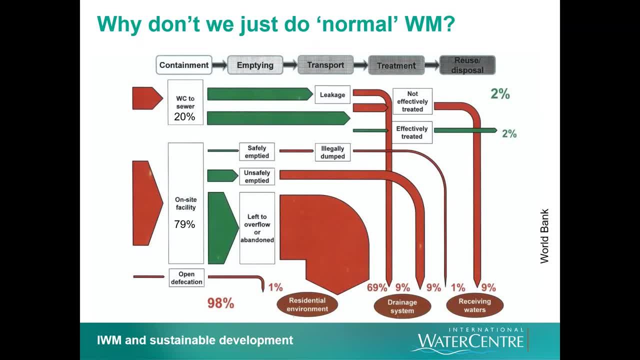 or objectives and policy formulation or strategic planning, when we're designing and figuring out what infrastructure investments to to make what, why not? why not just do normal, in inverted commas, water management? the slide you've got in front of you shows one of the reasons why not. normal water management involves water. 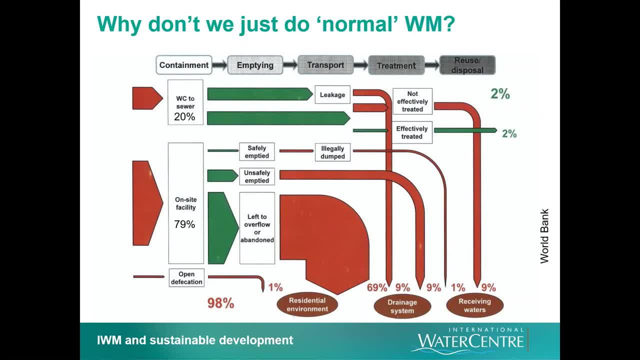 management problems, such as providing improved sanitation to an urban population, in this case, dhaka and bangladesh- being split up into parts and you'll see that top line. so the parts are containment, emptying, transport, treatment, reuse and disposal, in this case, if they form the it's. 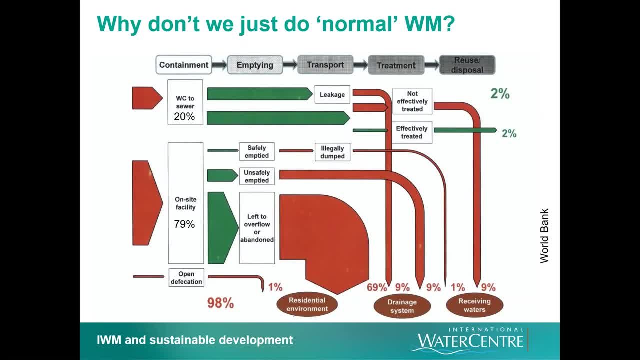 the parts of the sanitation chain. this diagram is is an example of our world bank sfd. sfd stands for ship flow diagram, and it's it's a way of mapping out what happens to to to solid- uh, well, liquid and then solid human waste. what this, uh, this sfd for dhaka, shows is that if we 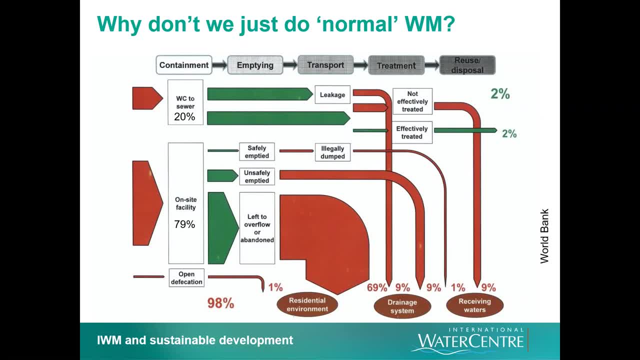 focus on one element and on improving it, for example, on improving containment. um, we, we, might. we can end up concluding incorrectly that we'll succeed. so in dhaka, this might mean seeing 99 containment of uh, 98 containment of uh- sorry, it's 99 percent containment of sewage- as having been 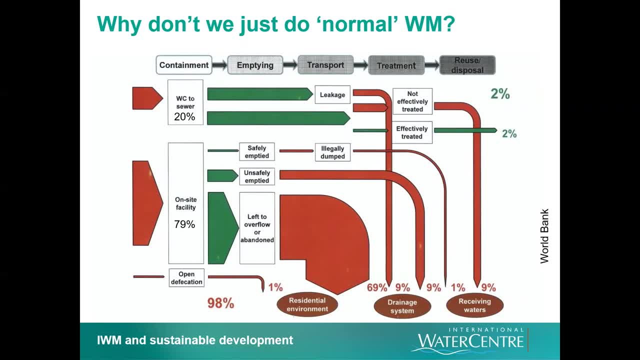 achieved uh. but if we stop to look uh, i suppose if we stop looking at the parts in isolation and chain uh, and how sewage and solid uh, biosolids uh, flow through it, then we can see that ultimately uh, actually only two percent. that's the green line that ends up on the right hand side. 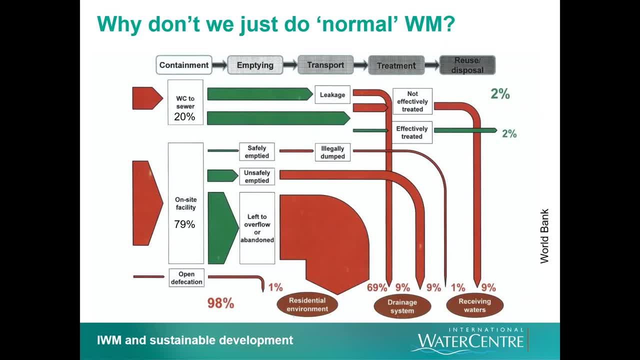 uh of sewage in dhaka is safely disposed of, 98 of sewage is not, and that means uh. it's a qualitatively very different conclusion from uh only examining the containment side of things. so we've got to. i suppose what this diagram methodology of the world bank is putting forward here is that we've got to think and act to. 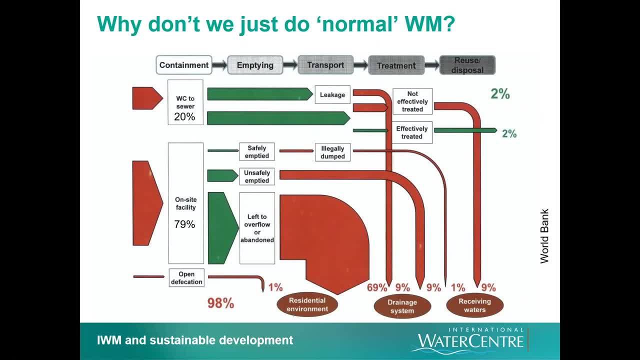 improve, i suppose, whole systems, um, and not just the parts of of systems, and unless we understand what the system is, it's very difficult to know whether we're improving the whole system or whether we're just improving some part but actually possibly causing more problems elsewhere. another example of a of why we don't just do normal, uh, water management. 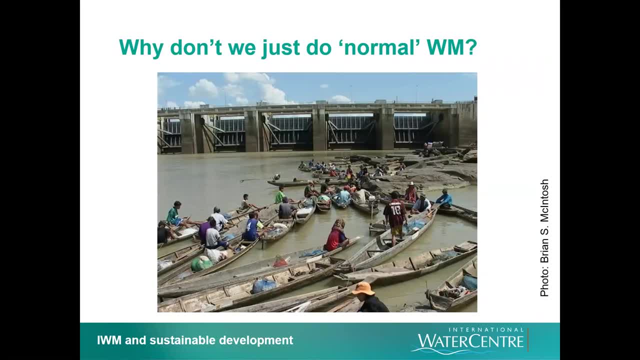 is the pac moon dam in front of you. this dam was one of the first dams built on a major tributary of the mekong in the mid-1990s and the. the tributary is the moon river in thailand. it joins the the mekong um uh at a town called kong gm. the dam was built to provide about 120 to 130. 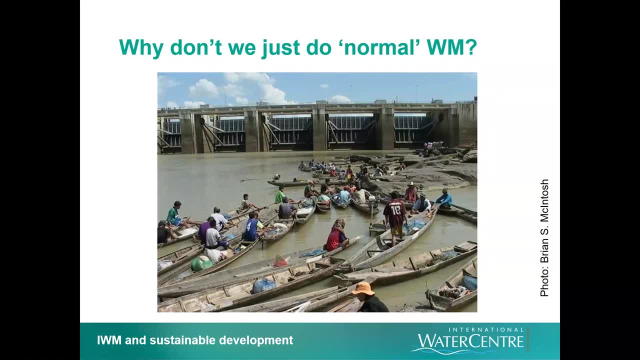 megawatts of power generation capacity and the engineers who who designed the dam, they didn't factor in the fisheries of the moon river um, fisheries which have provided the main source of protein and livelihood for thousands of people in isan province, which is the province in uh that uh the mekong um flows through, uh in northeast thailand. 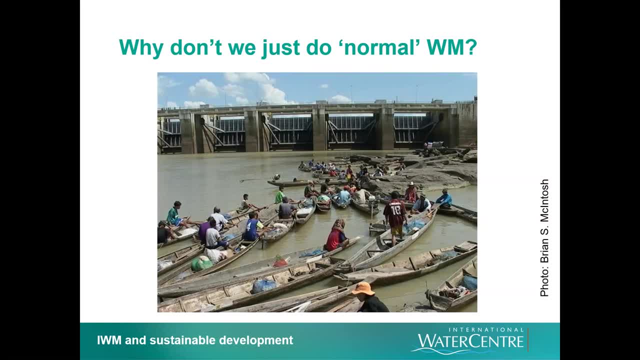 and they also didn't factor in that the fish and the in those fisheries require migration to to reproduce. so when the dam was built, uh fish were not able to migrate properly and around about 160 or so species from the 270 uh fish species in the river were effectively knocked out in terms of 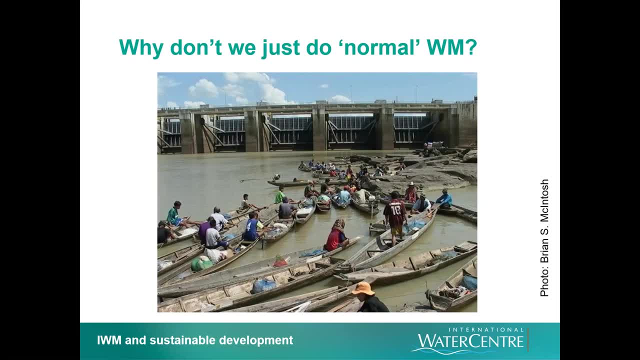 viable populations. this had the knock-on effect of disrupting the livelihoods and culture of of the villages on the moon moon river, which had been in place for at least 3 000 years, the the particular kind of subsistence and livelihood culture, and a disruption which um in combination. 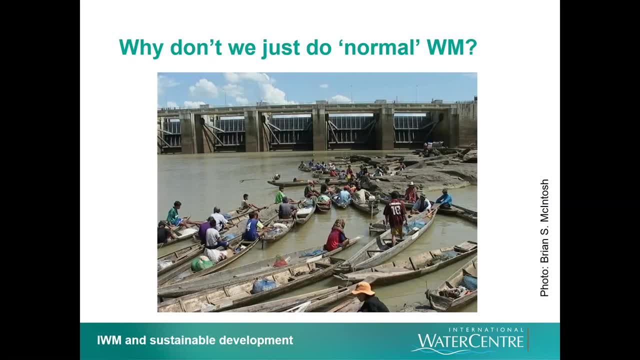 with other economic forces, including globalization, is it's still playing out in terms of changing village life near the the moon river in in quite fundamental and profound ways? um ways which you raise all sorts of questions about sustainability. um questions about sustainability such as: where do people get their protein from, now that they're not getting? 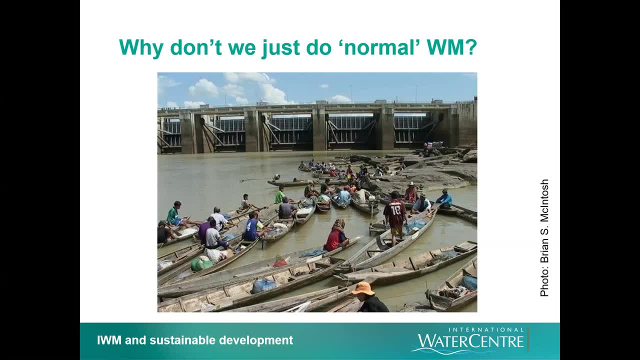 them from the river um stuart or from wwf released a paper a couple of years ago looking at the, the impacts and implications of of protein replacement. so if you're not getting fish from the, your protein from fish from the river, you're not getting fish from the river you're not getting fish from. 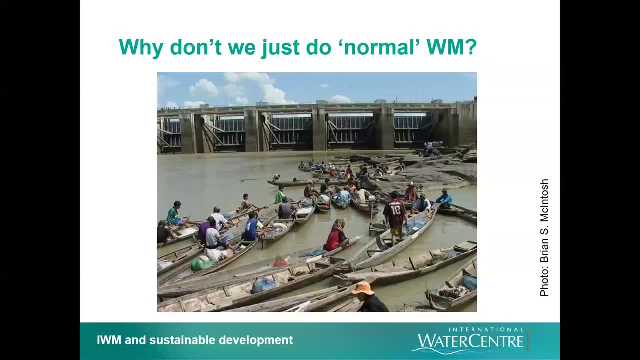 the river, which, in a sense, is free protein. you don't need to farm it deliberately. um. well, where else might that protein come from? and at the scale of the whole mekong, the uh, the consequences are are significant in terms of land clearing, um, which has, uh, both a water. 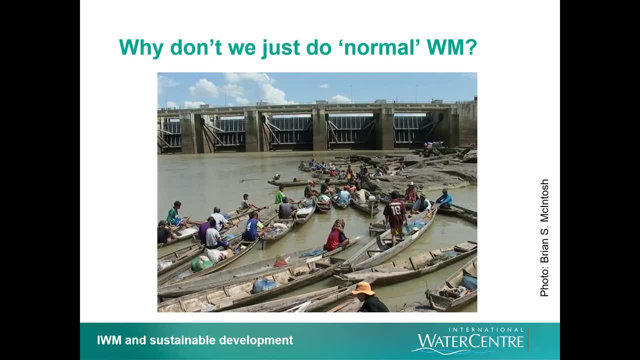 waterway health impact, a biodiversity impact also as a carbon impact. and then you've got to start intensively farming, and intensive farming requires energy inputs which are carbon emissions, nitrogen and phosphorus applied as fertilizers, which then have further ecosystem degradation effects. so the, the the regional, um, and down even at the uh, the local level, sustainable development impacts of. 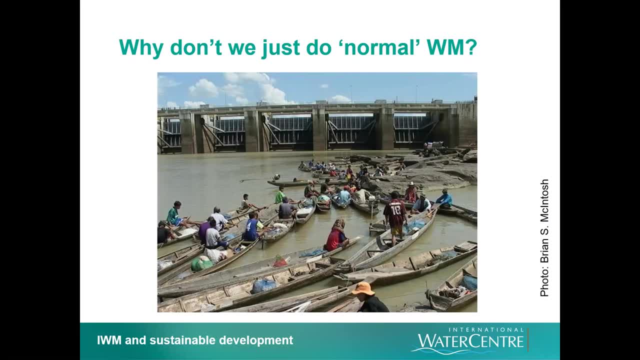 of treating energy generation separate from everything else, uh, have not been good, um, and have been quite profound and are still still playing out. normal approaches to water management don't emphasize looking out beyond the silos that are made from the ways in which we are going to. 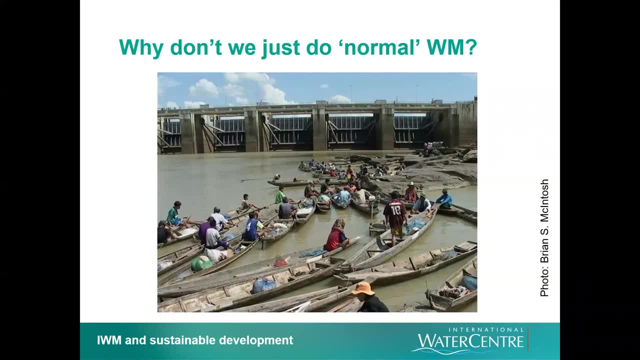 organize and structure and deliver water management. you know we've got to form organizations, organizations, we've got to do things. but the scope and the responsibilities of those organizations create silos which don't necessarily then coordinate with each other. looking out from those silos to inform policy planning and management from a whole of system, triple bottom line full. 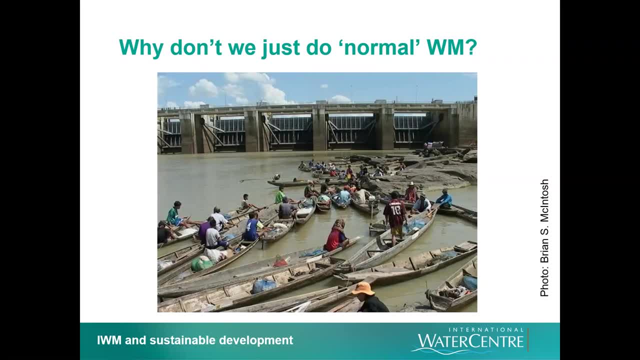 cost benefit perspective is needed really to ensure that we don't solve problems like not having enough electricity at the expense of creating new problems, such as the dirty water systems, such as the degradation of fisheries and livelihoods, and the need to to then put in place um very energetically and environmentally damaging um alternatives to, to protein production, and we can. 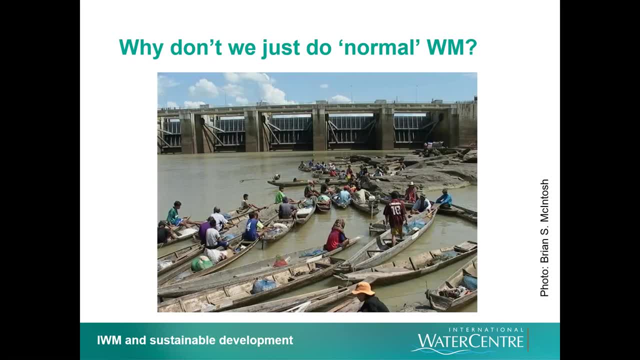 think of such practices as problem shifting. uh, and potentially resulting in uh. we can. i suppose we can think of such practices as problem shifting. so normal water management runs the risk of shifting problems, of of creating net costs rather than benefits. you solve a problem in one place and you 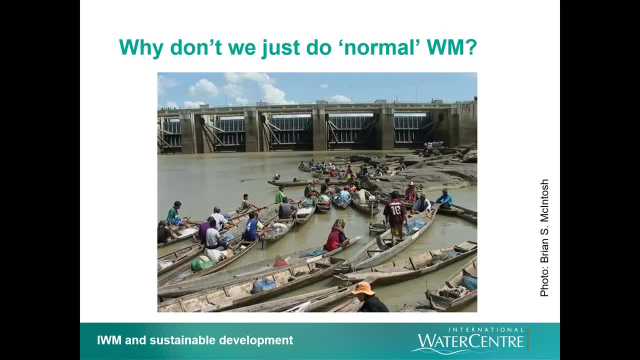 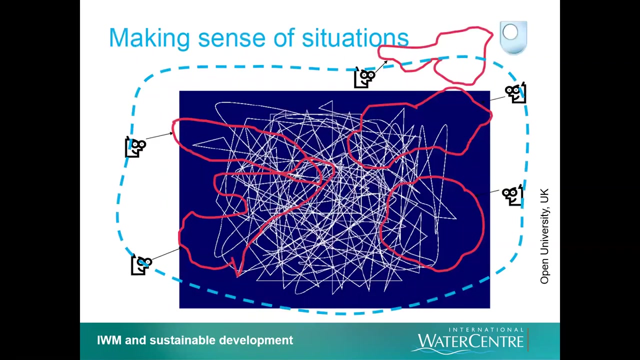 settle problems elsewhere or downstream um, and you change the the distribution of costs and benefits and risks across stakeholders and not necessarily in good ways. and one of the problems is, i suppose, normal water management in complex situations is that quite often you don't know what you don't know um. i suppose iwm starts from a position of accepting that it's not possible. 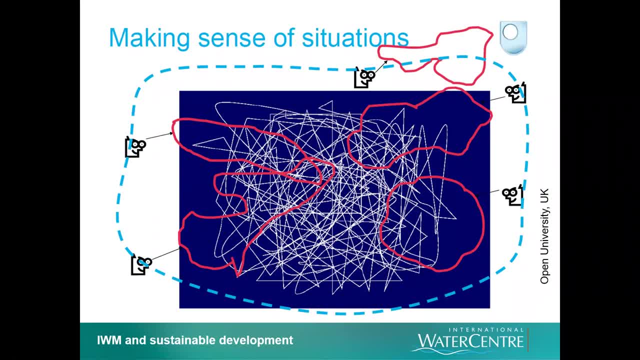 for any one person or organization to fully appreciate a situation. and a situation might be a village, might be a whole catchment, might be part of a river. if it's a whole of a catchment, it may be small, it might be large, like the like the mekong. 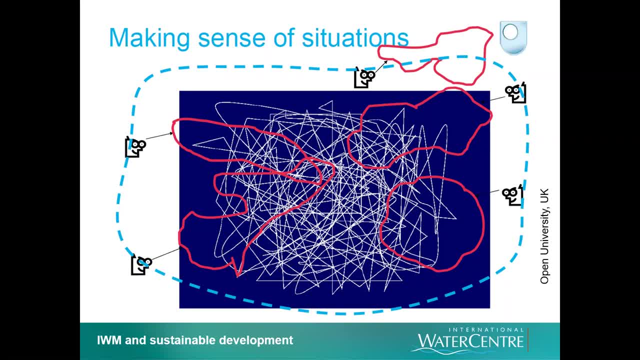 it might be a city and a situation might even be an organization. the kinds of situations that probably motivate all of you- and the kinds of situations that motivate me are- are complex. um, this is a great diagram from the open university in the uk and it sort of shows a complex system as 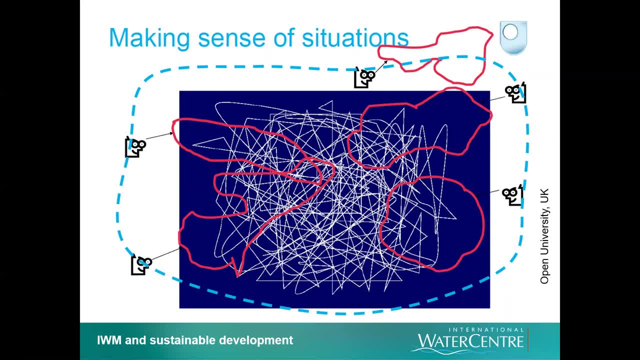 being a bit like a really large bowl of spaghetti or noodles: um, that's moving around as it's being eaten. um, it's, it's too big and it's moving and, as a consequence, it isn't possible to see or know everything that's happening. um, so that's what you see when you've got those little heads. they 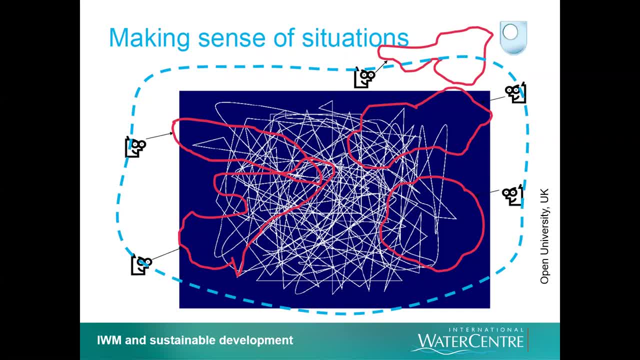 represent us people, individuals, looking in, uh, sometimes actually from within a situation, sometimes from outside, and thinking that we might see everything. but of course we don't, uh, and we're quite often unaware of the the bounds of what we're seeing and what we're not seeing, and we're quite 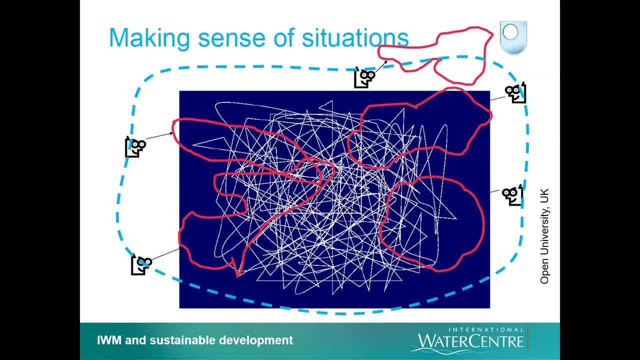 often unaware of the, the bounds of what we're seeing, and we're quite often unaware of the, the bounds of what we do know and what we don't know. um, it isn't possible to see or know everything that's happening, and our individual and cognitive and value-based perspectives limit what we see. 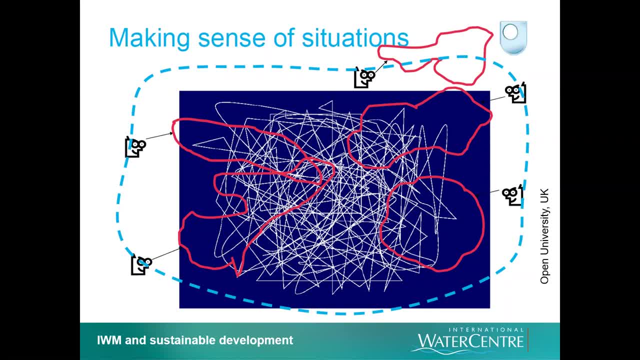 uh and sometimes uh forces to unconsciously to, to filter out things you know where. we just don't see that it's important, so we don't pay any attention. iwm um, for us at the iwc starts from the position that we cannot work in silos, that we cannot necessarily comprehend the the kinds of 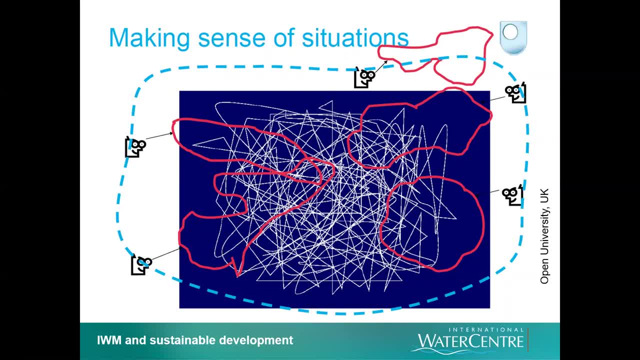 situations in which we work, uh, and we must, as a consequence, reach out to others to ensure that we're able to bring the sufficient diversity of perspectives to the water management or sustainable development situation at hand. this view frames iwm, i suppose really is being a rational response to the inherent limitations of complexity, complexity which exists because 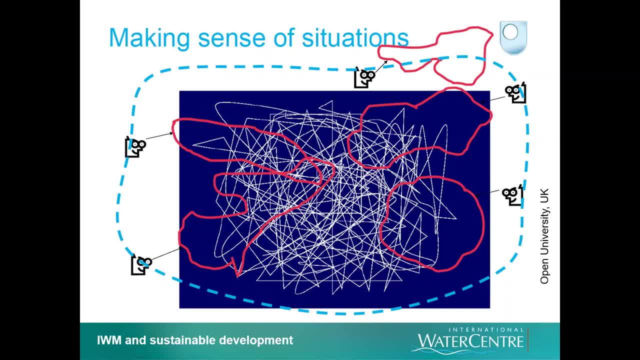 we work in situations that are comprised of often hidden social, ecological, hydrological and economic and impact capacity and uh, and so I think in shirley's uh continuouslyında come ribss and situations where there may be different diagnoses of what's wrong and therefore what. 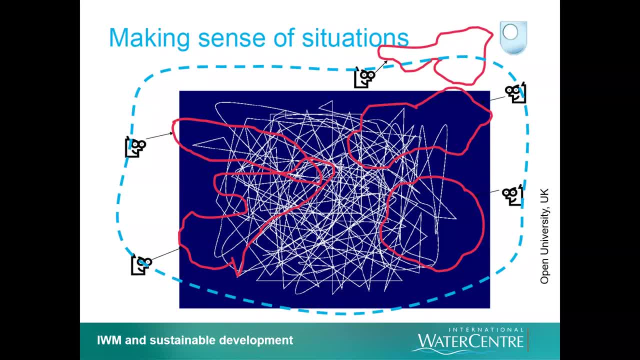 should be done. Such situations are, I suppose, what are certainly complex and they're quite often called wicked, or those situations present wicked problems. The Pacman Dam engineers- to briefly return to the Pacman Dam, they wouldn't have deliberately intended to degrade fisheries and 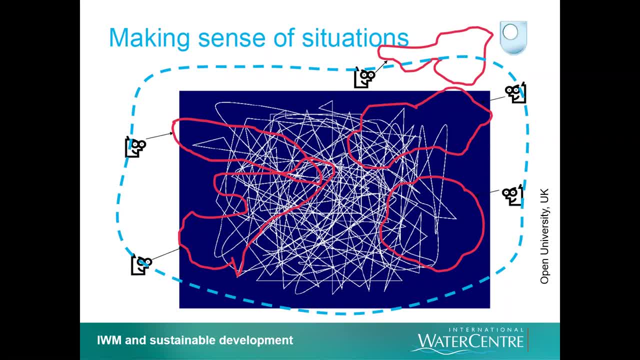 livelihoods. I've got great faith in people not intending to act badly, but, more likely, they simply did not know that the dam would have those impacts. They were caught in a silo. They were caught, in a sense, in a cognitive trap created by the roles and responsibilities and the 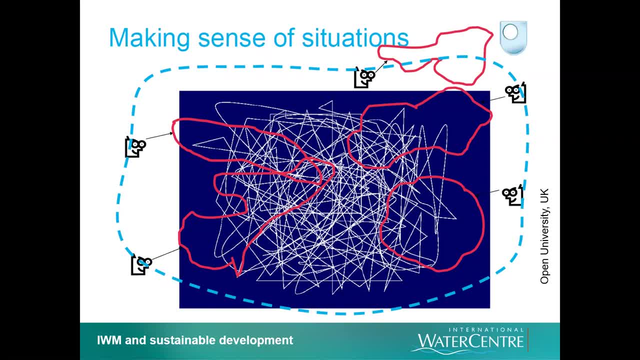 bounding of their organisation, plus their own disciplinary cognitive biases, They were caught in a silo, planning how to generate electricity without even knowing that they didn't know anything about the the wider context. An IWM multiple perspective approach could have avoided this. So, seeking and 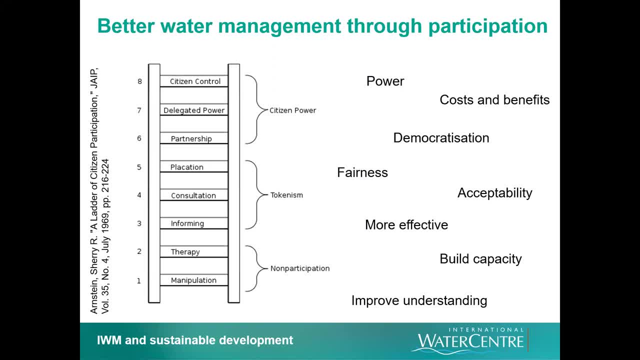 engaging with alternative and multiple perspectives is perhaps, then, key to the practice of IWM. It offers a way to uncover the aspects of a situation that you don't know you don't know, and to incorporate their consideration into whatever it is that you're doing: policy planning management. 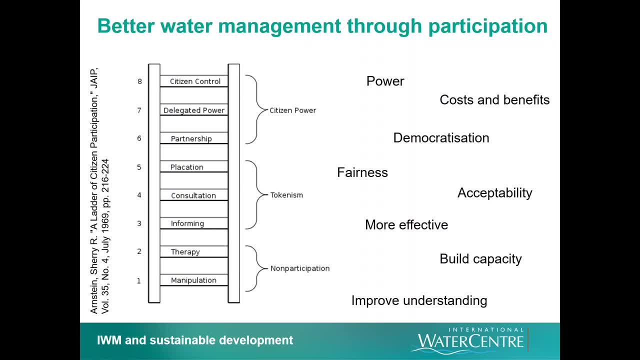 This is, I think, a rational and a pretty practical response to complexity. You know, you don't just say: oh wow, it's complex, throw my hands, don't amazing, don't know what to do. Actually, you can do something, You can collaborate, you can participate. It's also a way of 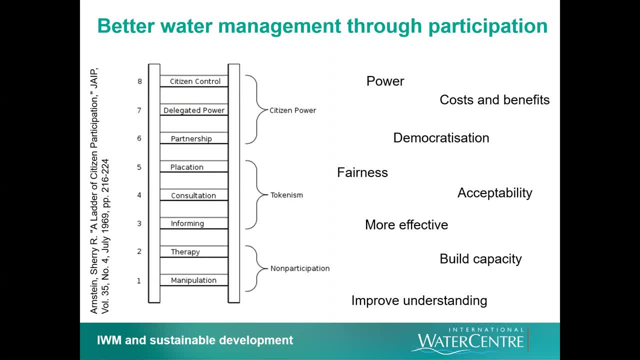 ensuring that the implementation of sustainable development provides a mechanism for dialogue and deliberation across stakeholders. And remember that sustainable development, despite the clear framing of the SDG's, is contested. Not everyone's necessarily going to agree with what the SDG's have put forward as as being the 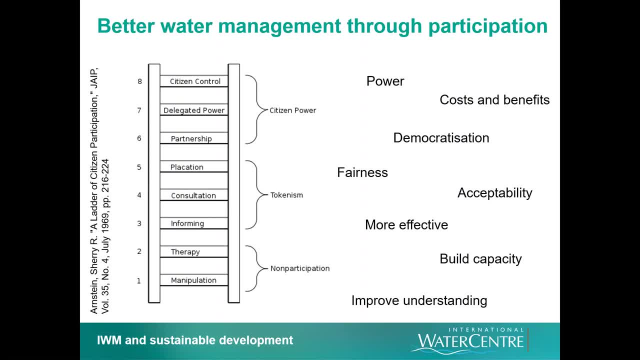 clear framing of the SDG's is contested. Not everyone is necessarily going to agree with what the SDG's have put forward: las being the Reliant on the development of sustainable projects, a very comprehensive award, andzhou marque. One of them was the article that we asked the Wellbeing within the consortium for branding what SDGs are funds. They were at the lower end, SEHDU as well, for perception of a 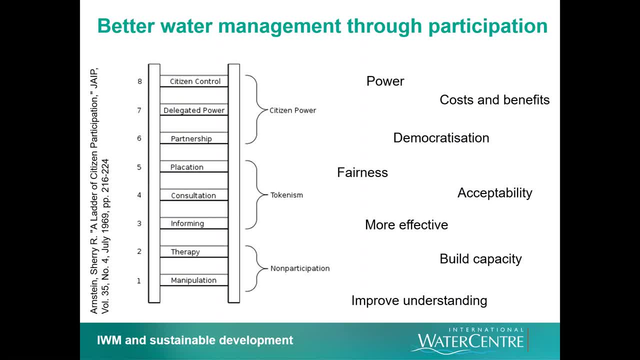 have put forward as as being the the key priorities and the ways of measuring the achievement of those priorities, and the fact that it's contested is: is that's fine? you know that's about complex situations, which are partly complex because people have different views as to what's going on and what should be done, engaging multiple perspectives as we collectively decide. 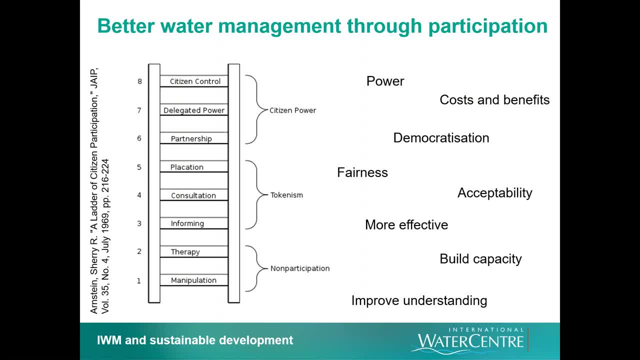 on the direction and navigate towards, somehow towards sustainable development can be done through participation. this can involve including ordinary citizens or communities and decision making in planning processes. participation can be thought of as having a range of levels, from less to more, from manipulation at the bottom, which is not so good, to citizen control at the 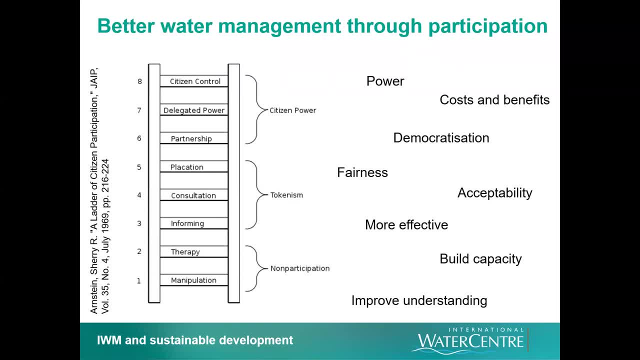 top which might be viewed as good, but as a set of practical problems in terms of cost and time, as shown here in a. this is a sherry Einstein's famous ladder of participation and came from her paper which is referenced on the left-hand side. participation, as well as helping to uncover the things you don't know you don't know also provides a set 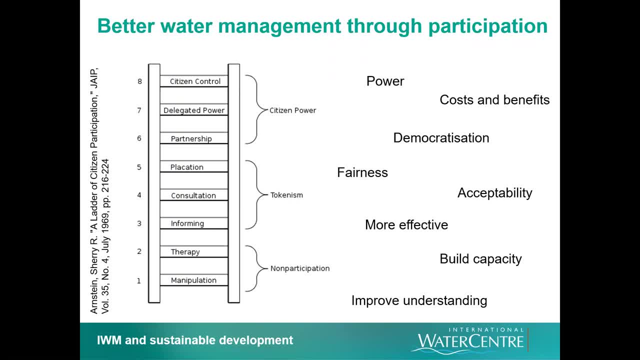 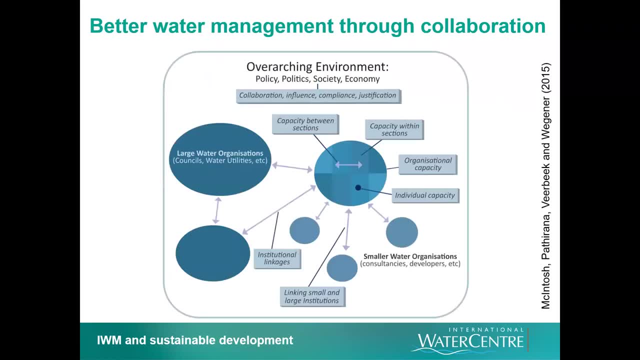 of benefits such as democratization, fairness, capacity building and potentially also increased levels of acceptance and effectiveness for for management actions. multiple perspectives can also be brought to bear by collaboration across organizations. the diagram in front of you comes from one of the most recent papers published in the United States by the University of New York. 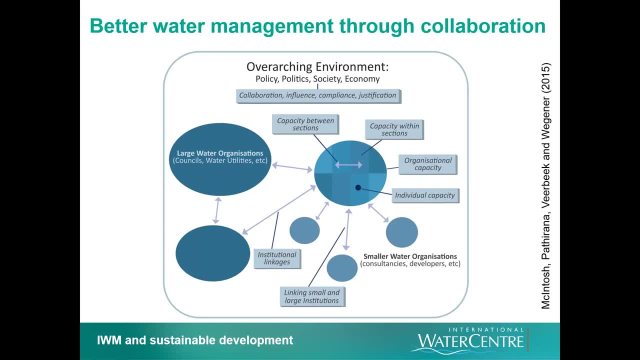 on the work that we did here at the IWC about how to transform urban water management to achieve a set of sustainability dimensions and ambitions, which were wrapped up in this thing called the water sensitive City. the work that we did emphasize the need to build capacity both within and across. 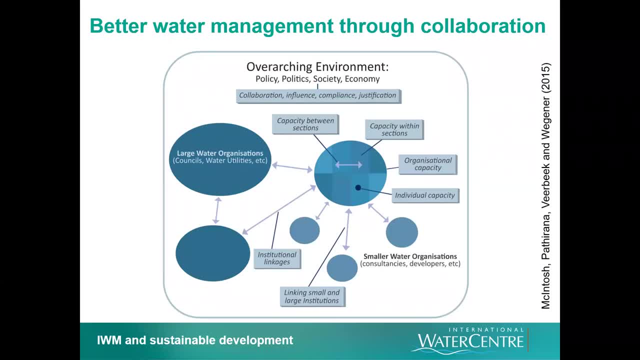 organizations responsible for different aspects of the urban water cycle, from water supply and sanitation through flood risk management to public green space planning and maintenance. building capacity across organizations is about, for us at least, about building capacity to collaborate, to understand the remits and objectives of other organizations and maybe even other departments and teams within your 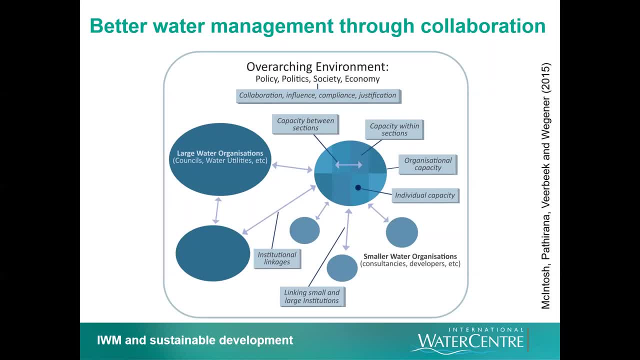 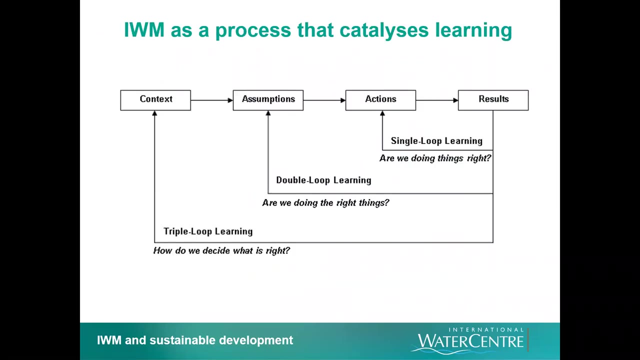 organization to generate trust- trust is what makes collaboration possible- and to become able to see how to work together in new and perhaps unexpected ways that have got benefits win-wins to. to both parties being concerned with incorporating multiple perspectives in order to take a whole of systems approach to improving situations. 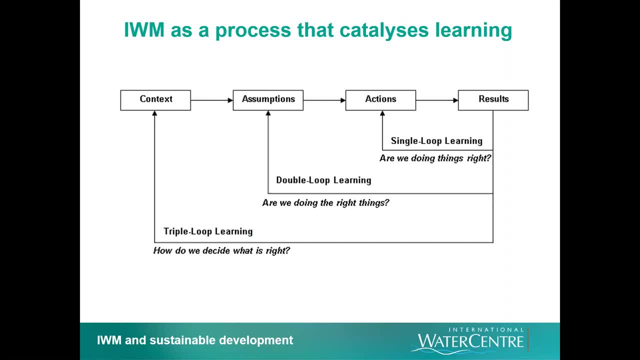 that's certainly what we view IWM is being- is really at its core, it's about. it's about learning. it's about learning, but not so much about how to get better and more efficient at delivering water management outcomes in traditional ways, what we may and what you'll see in the diagram there being 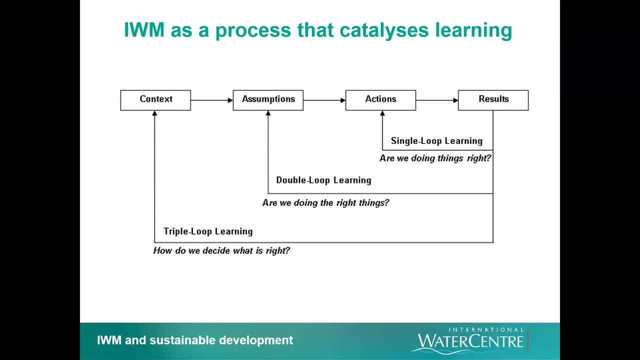 as called single loop learning, which is: are we doing things right? you know, are we? are we reducing the costs? Are we getting better at delivering X or Y? Rather, IWM is about a different kind of learning. It's about catalyzing learning across perspectives, which then creates opportunities. 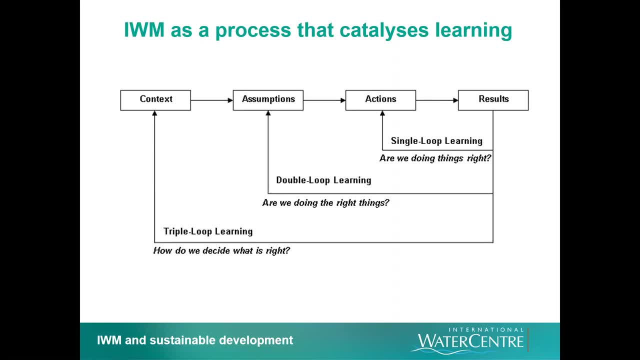 for double-loop learning: Are we doing the right things? You might be doing the wrong thing very well. You need to have processes and opportunities and ways and mechanisms within the organization that you work in, across organizations, to pose this question: well, actually, are we doing the right things? Maybe even to pose the question: well, how? 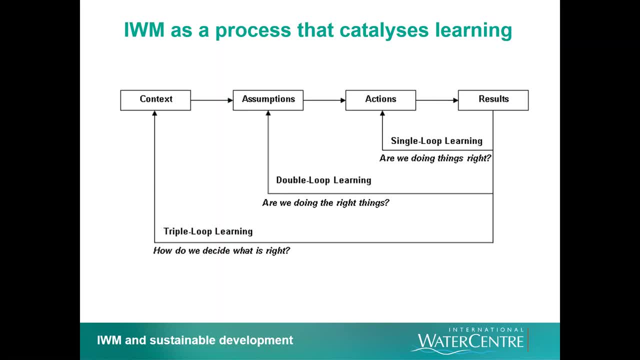 on earth. do we decide what's the right thing to do here? Realizing that current practices may not be adequate starts such a process of learning, which then creates the way in which new ways of doing things might be developed, new ways that might address new drivers or 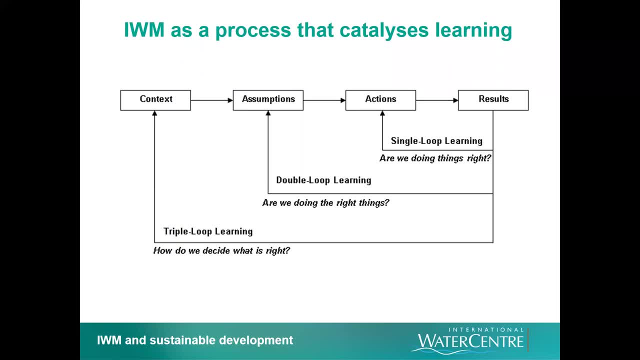 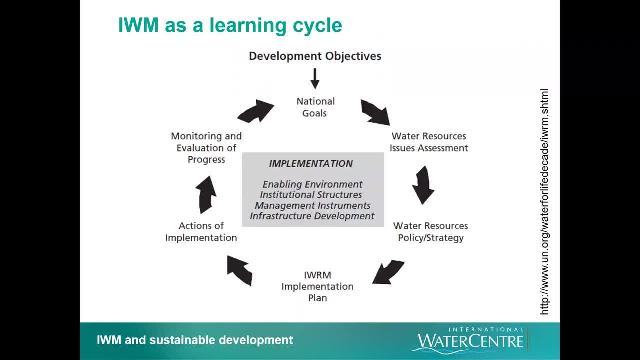 the process of learning. It's about the process of learning. It's about the process of learning. You might think about them being more than a fixed set of steps in a process that implements IWM. Perhaps I suggest that you might think about them as a set of steps that create opportunities. 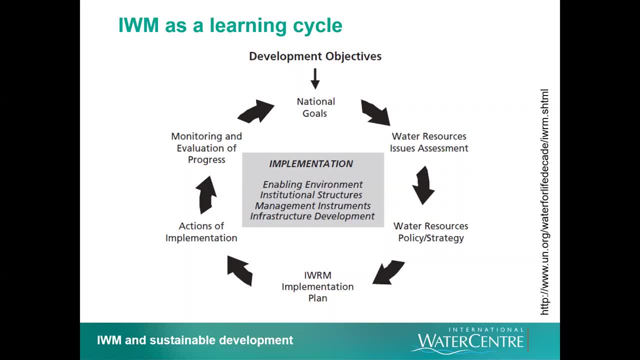 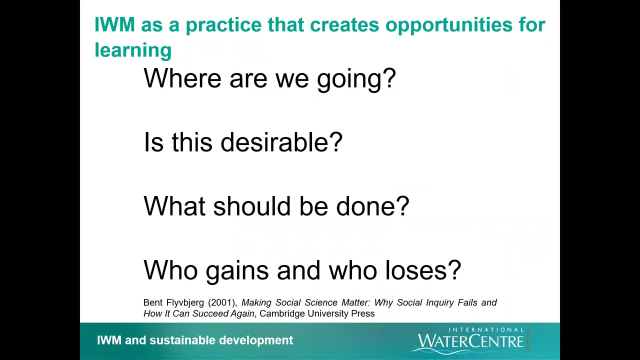 for learning about the direction that should be followed to implement sustainable development, and a set of steps that provide opportunities for then figuring out how to actually move in that direction. So how might we manifest IWM as a practice? Well, there are opportunities every day, Whether you're in a project planning or management meeting, whether you're having a conversation a bit more informally with members of your team, whether you're in longer scale program planning. 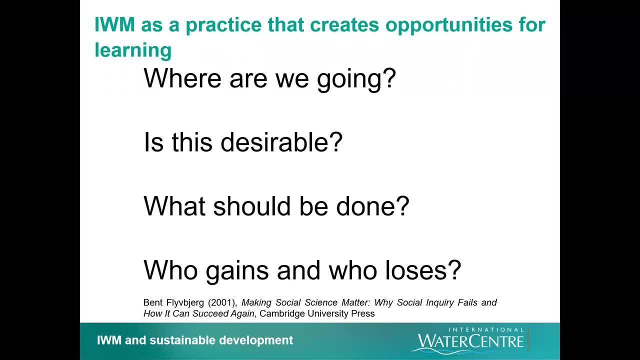 And these opportunities need to be created by people, people like yourself. They are opportunities to. they're supposed to start conversations about whether the right things are being done or not, And those kinds of opportunities can be created by asking pretty simple questions like the ones on the slide. Of course, you're not going to ask them in, perhaps in exactly the same form as they are on the slide, and you're not going to ask them all the time or all four of them all at once. 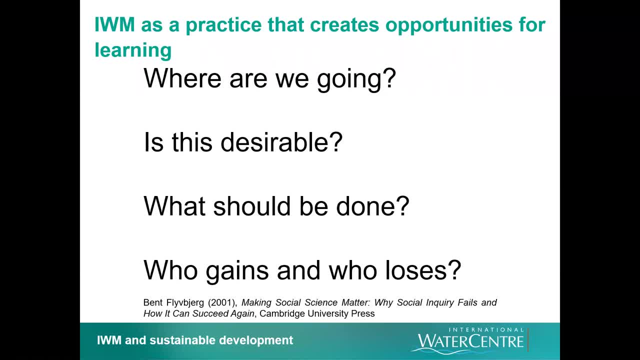 People will start to think you're a little bit crazy in your team conversations, But you know, using these questions, plain, simple English questions: where are we going with this, Is it desirable, Who's going to gain and who's going to lose and what should be done? Pretty easy questions, Easy questions which create the opportunity for the people that you're talking with to reflect and to engage in learning, which might then open up that double or triple loop learning. 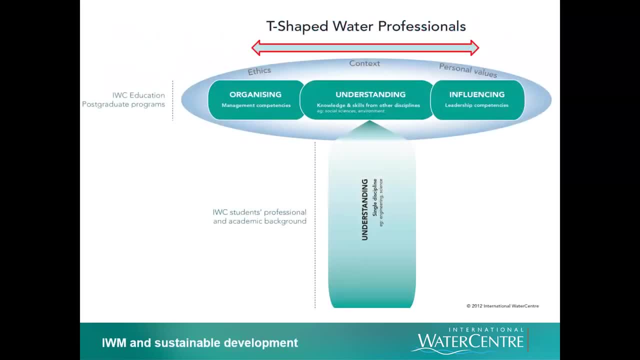 Process At IWC. we think that to engage in such conversations across multiple and diverse disciplinary, functional and community perspectives requires a particular set of skills: Skills and being able to understand and translate what you hear into your own discipline or function, so that you're able to identify ways of bringing together multiple objectives from multiple stakeholders and views. 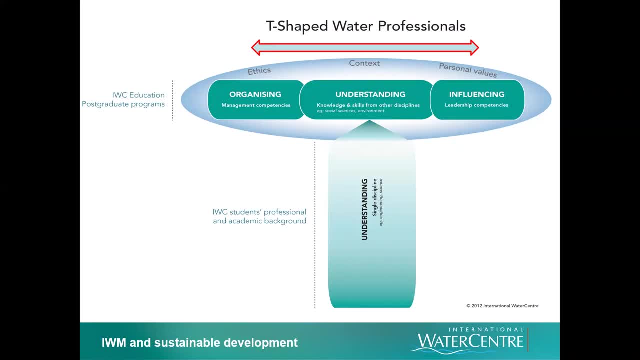 We think of these skills as being a kind of a profile, A T-shaped profile. So if you look at the screen, there's a T in front of you. If we think about the vertical part of it, it's the eye. So we have deep, the vertical dimension knowledge about a restricted scope. That's why the eye, the vertical bar, is narrow. 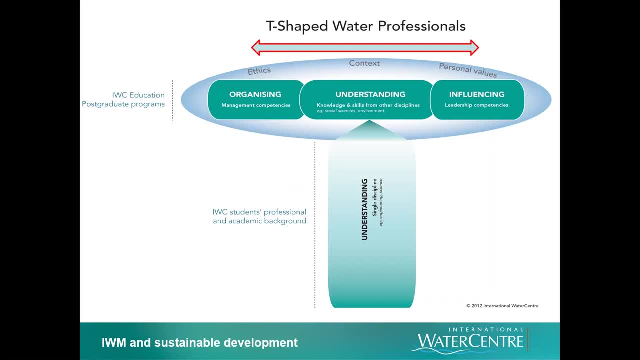 And we think that a T-shaped profile is composed of deep specialist knowledge. So an engineer knowing a lot about civil engineering, for example, complemented by a crossbar, And we think that that's a T-shape, which means then that that engineer, for example, is able to talk coherently with an ecologist, or with an economist, or a lawyer or a community development practitioner. 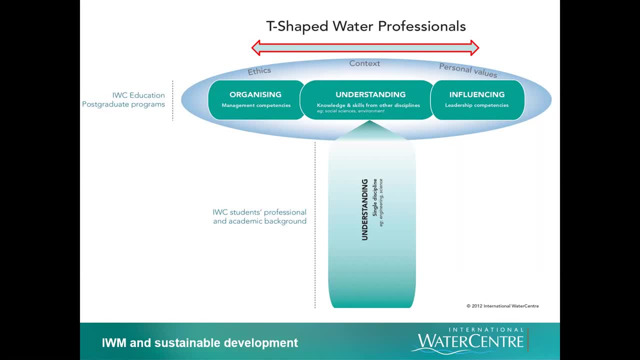 And they're able to figure out how to incorporate that other person's objectives into their own. Water-sensitive urban design and water sensitive cities, as I suppose is an example of sustainable development in urban form planning and water management to some extent has come about as a consequence of engineers learning how to how to talk with. 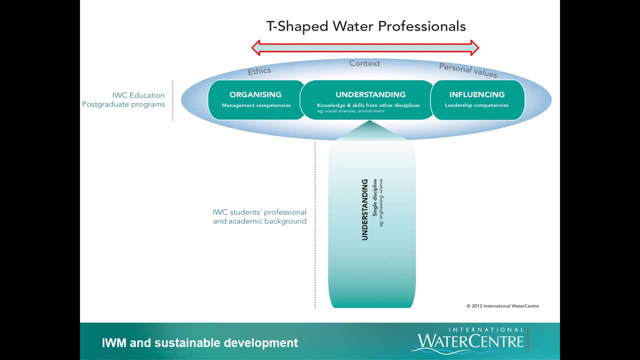 others learning. actually, from an ecological perspective, draining water out of a city really quickly is is not a good thing. it causes erosion and degradation of stream, channel form and ecological habitat. actually be much better to slow the water down, so engineers can then think about how to manage flood in a way that that that that doesn't cause ecological degradation. 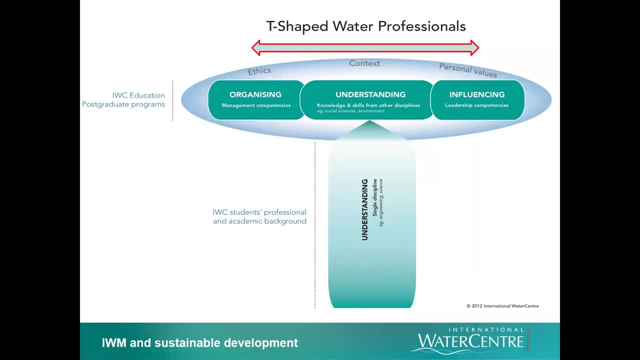 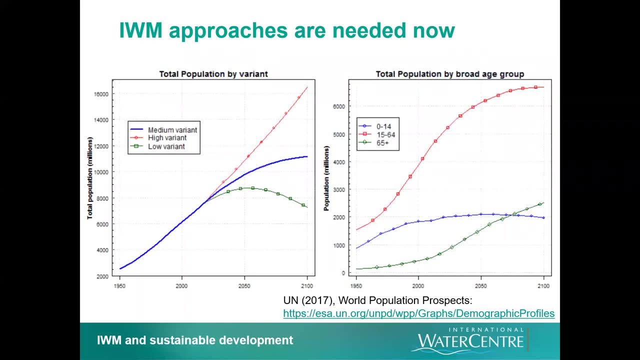 and that only happens if- if you have engineers willing and capable to talk with ecologists and ecologists willing and capable to talk with engineers. we. we see that this sort of need to, to, to act collaboratively, collectively and whole of system scalers is is pressing. we see that we. 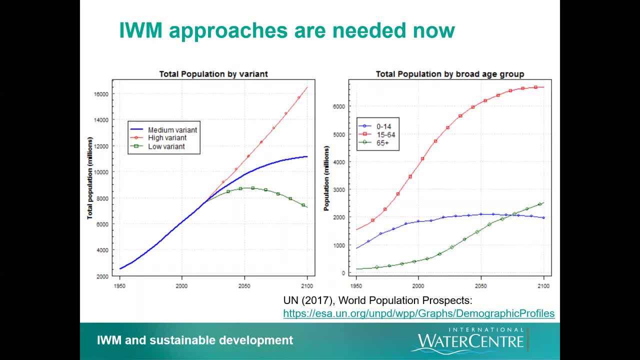 there we see that we need to to collectively develop the capacity in individuals, organizations, sectors and across sectors to engage with each other and to start the conversations that will ultimately lead to changes in the way that we we think about and manage water. we need to do this because we we have really fairly significant 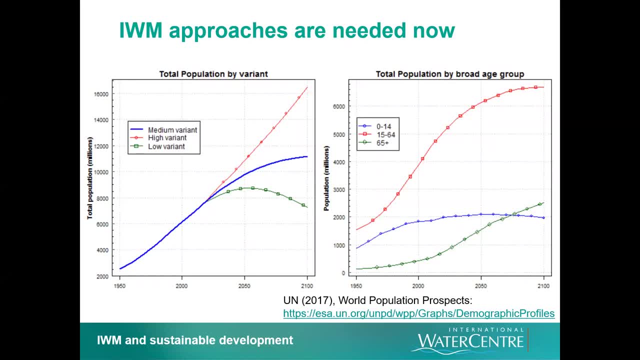 challenges in the 21st century. we have a set of drivers which mean that our countries and the world overall is is really under pressure like never before. there's no more than 7 billion people in the world, and we need to do this because we have really fairly significant challenges in 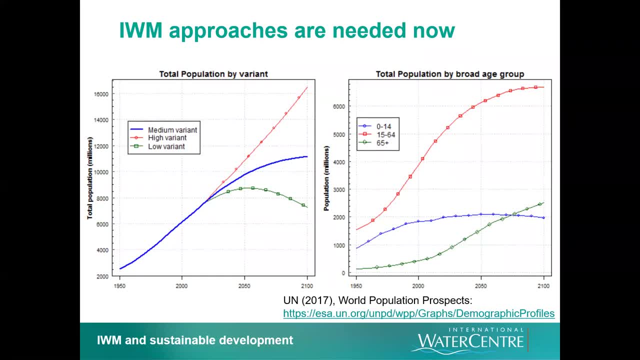 this context because we have really pretty serious challenges in climate change andGS. one of that- Yeah, has always written reply helps to the us to get the breathing of Venezuelans come to study. 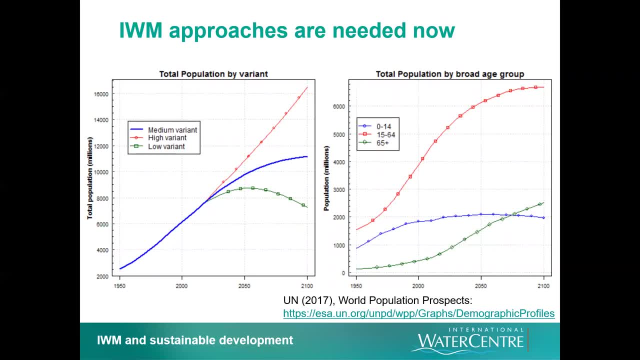 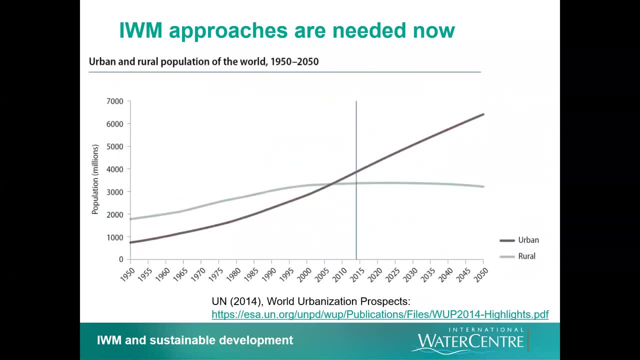 demand for water, for sanitation, for food and for energy. We also now have most of the world's population living in cities and this creates problems, but it also creates opportunities. Problems in that urbanization and the disruption of catchments. 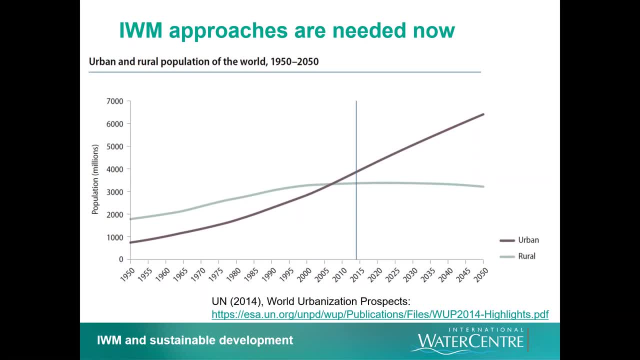 and then natural hydrological and ecological processes is severe and widespread and growing, but also solutions and perhaps that we can, like the water-sensitive city ambition, perhaps more cost-effectively service urban populations with water and wastewater. Perhaps we can create resource recycling loops. 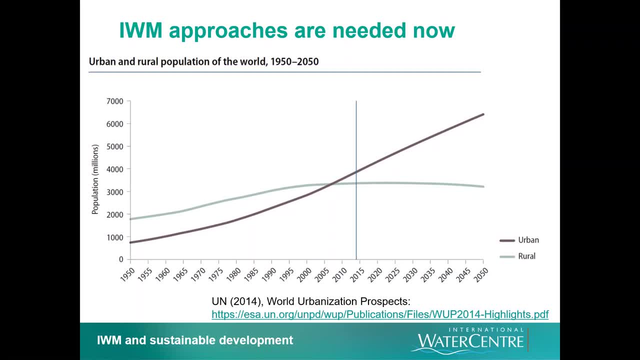 Perhaps we can manage floods and storm water flows in ways that don't cause, in fact to some degree actually restore natural catchment, hydrological and ecological function to cities. So we've got everyone working and living, more people living more closely together. 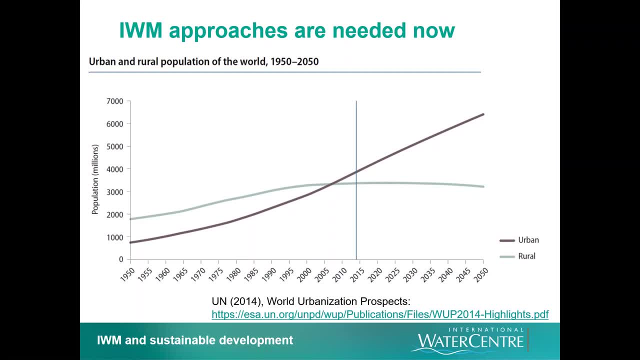 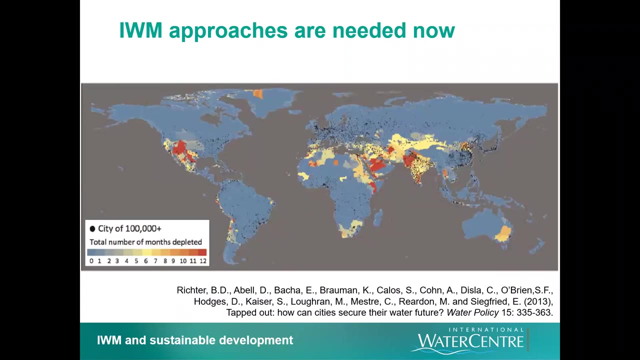 That creates the opportunity. That creates the opportunity for cost-effective investment, but only if we understand what to do through collaboration. Suppose we see that the need for collaborative systemic action is also pressing because we're already beginning to face water security constraints. So this is about five, six years old, this paper. now 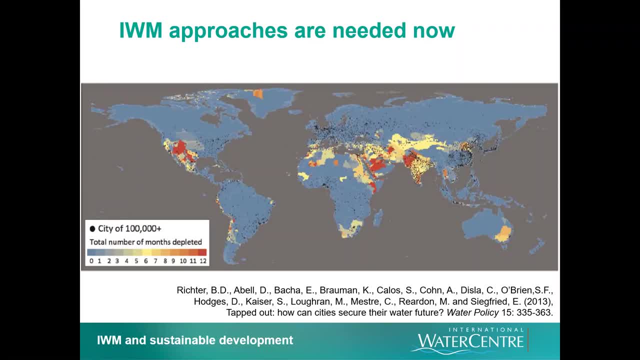 but the diagram in front of you shows the results of some analysis which were conducted a few years ago by Brian Brian Richter and colleagues. They took a definition of a city as being 100,000 people or more and they demonstrated that more than 50% of the world's cities 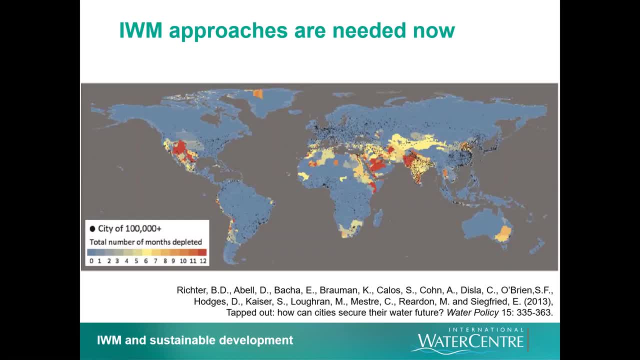 defined as 100,000 people or more are in river basins where net withdrawals of water are more than net inputs. If you add on the impacts of climate change to those basins, which they didn't do in their analysis, the outcomes will become more complex and likely more problematic. 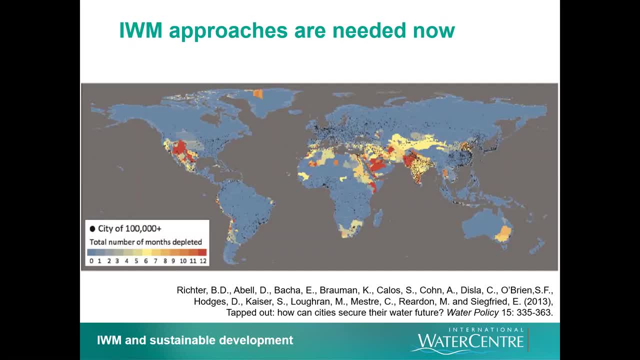 These cities. you know they're not going to run out of water tomorrow, but they have no long-term water security. So you might think of Cape Town in South Africa, but in multiple locations, potentially combined with significant extreme flooding and the oscillation between flooding and drought happening in much more rapid and unexpected ways. 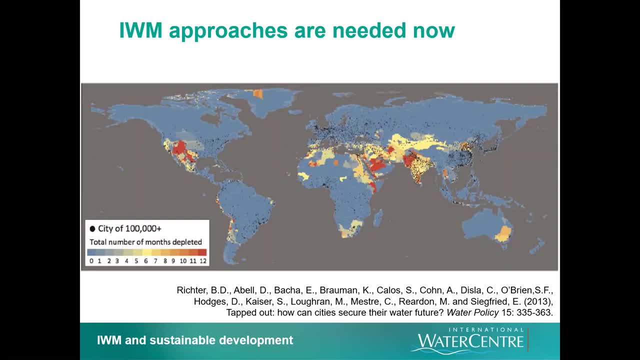 I'm thinking a little bit locally here. We we've just had significant extreme flooding which has happened about about a thousand odd kilometers north of Brisbane, where we are in Queensland, in a town called Townsville. a city called Townsville surrounding region went from a really severe multi-year drought to having a year of rain. 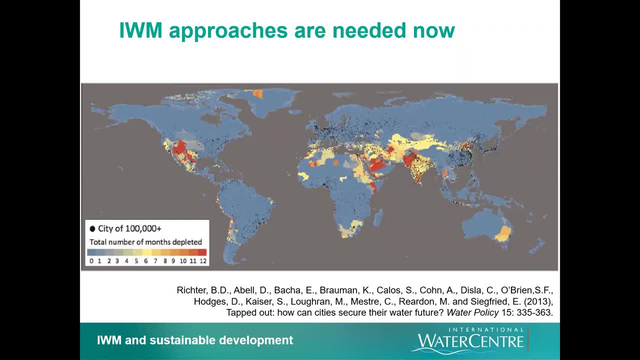 a year's worth of rainfall in a week. So we need to think about water security and in quite radically different ways. We need to think, we need to get out of our silos and start to act collectively if we're going to adapt and achieve whatever we think of as sustainable development, whether it's the SDGs or another interpretation. 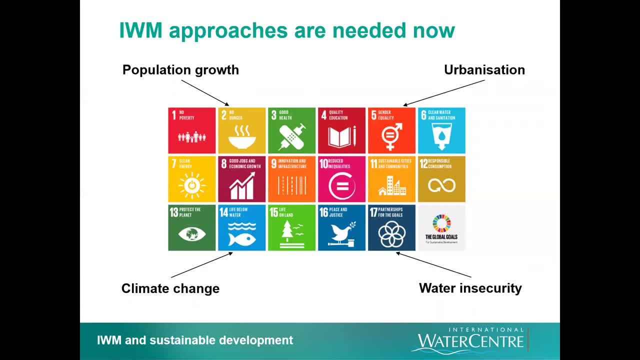 So look we've. We've come in this talk a sort of fair way from the SDGs. What I've hoped to have done is to have outlined a view of IWM as being a general set of principles and practices which respond to complexity by employing participation and collaboration. 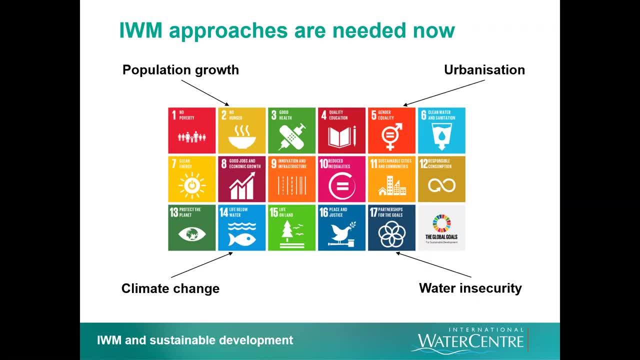 and employing them really for the purpose of learning from other perspectives about how to take better action towards this continually evolving aim and definition of sustainable development. So IWM for us at the IWC, in a sense, is nothing more than a set of skills employed by people in processes. 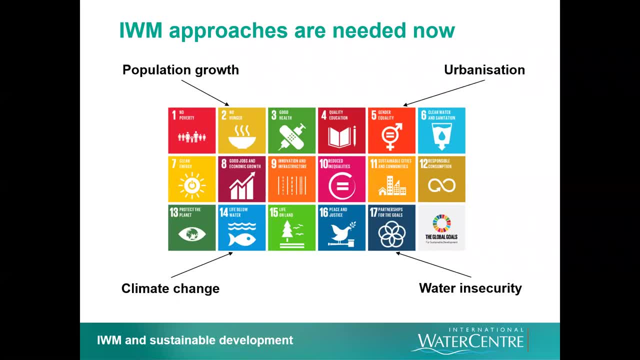 in organisations and teams across organisations, skills that can be developed really in anyone and which can be manifest in situations from strategic plan formulation to normal project delivery and design, to everyday team conversations at your work. We need, I suppose, to be able to identify. 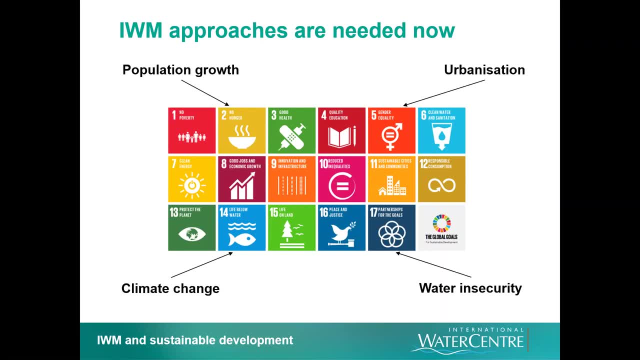 what we don't know. we don't know. We need to be able to work at the situation or systems level if we're going to stand any hope of achieving the SDGs in the face of population growth, urbanisation, climate change and water insecurity. 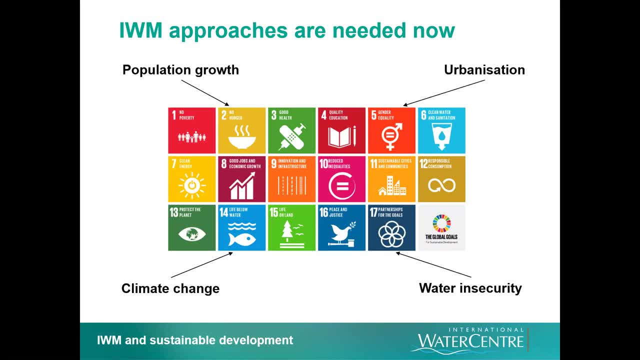 So I hope you've enjoyed this presentation and I guess some insight into our take on integrated water management and consequently also integrated water resource management. I'll leave the presentation here, but perhaps with a last word, that IWM skills and approaches are, from our perspective, really needed now more than ever. 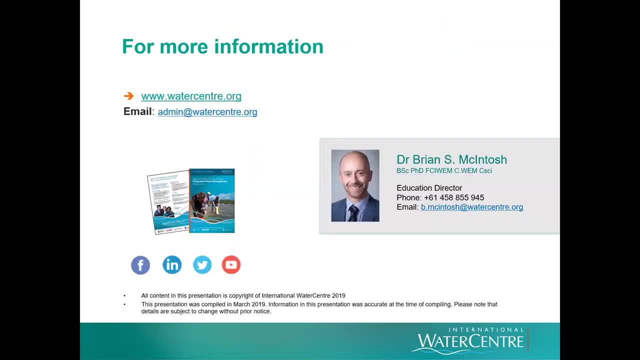 because of these multiple pressures- and I'm happy to take questions just now and also happy for people to contact me anytime- really, Visit our website, which is going to be relaunched. The navigability isn't that great just now. We are going to redo our website. 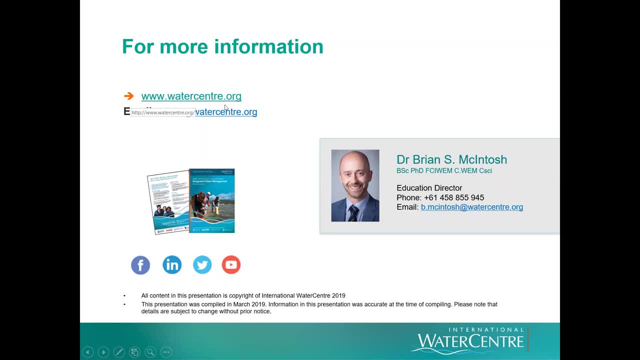 which will be up and running in about by the end of April or so. Visit our website. You can contact our general enquiries email admin at watercentreorg or you can contact me directly at bmcintosh at watercentreorg. And I'll stop there. 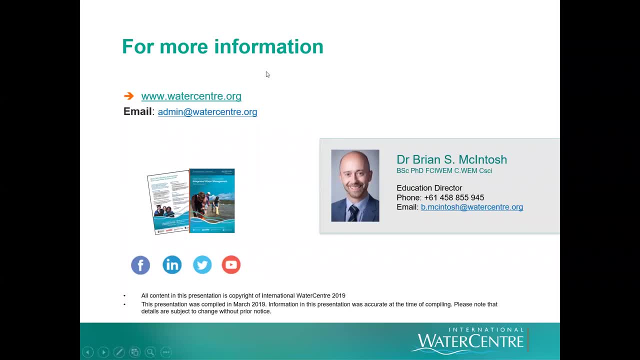 Perfect. Thank you, Brian. so much for this great and really interesting presentation. So anyone who has question can either ask in the chat or just raise a hand. I see quality in the chat and you can ask Brian directly if you want, And I for sure have enough questions. 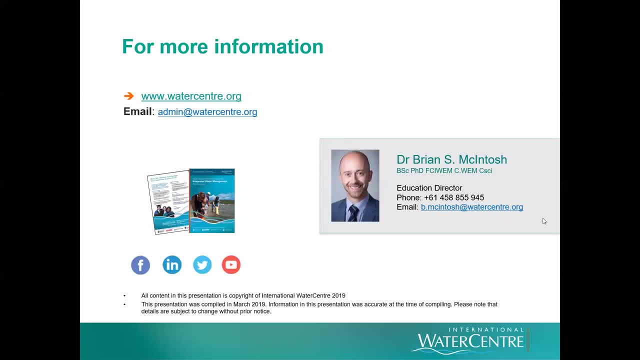 but if any one of you who joined us for this presentation wants to go first, No one right now- Edward Bornula- has said thank you, Thank you, I think it's Edward, Thank you. Cool, And then I would just start. 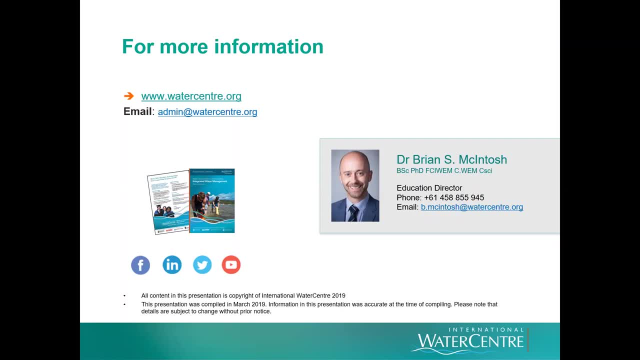 Maybe someone has to be the first to make some more. So I work mostly in climate change. If you say a big word, I'm just one scientist and a big problem and even bigger problem. But do you think we are able to solve problems and like reducing things we already do? 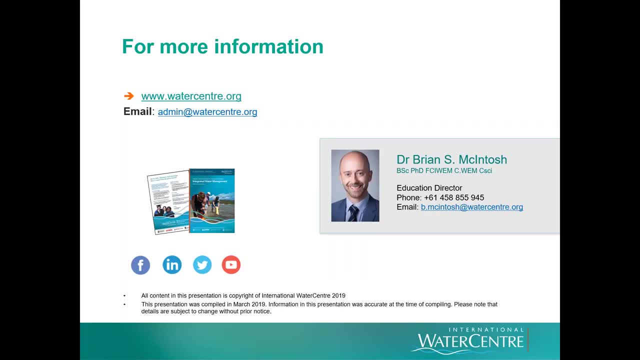 Or do you think the way is actually to go? stop what we are doing and trying to- how to say it- to not make it worse. So I think climate change- we can't go back, but we can make it slower or stop some things to not make it worse. 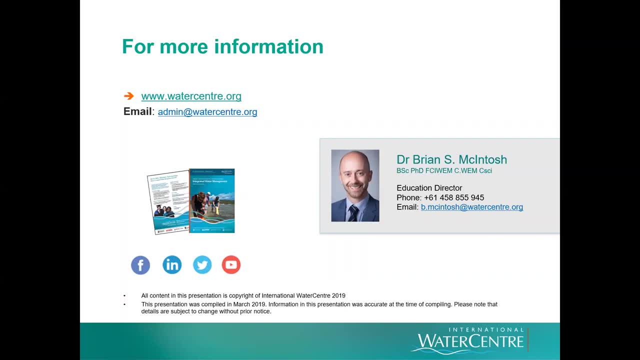 What do you think? with water scarcity and stuff like that? What is the way to go? Yeah, So I suppose you've got to. climate change is an interesting one, because it really is. It's a global commons which requires, requires some action, really from. 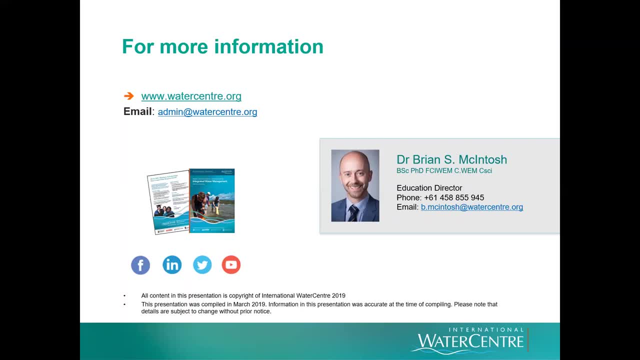 from from from everybody and from every country Water scarcity is. it's at least got a couple of different scales of action there. So from a systems perspective, what you tend to talk about is improving situations. So how might we improve the water security of a city or a region? 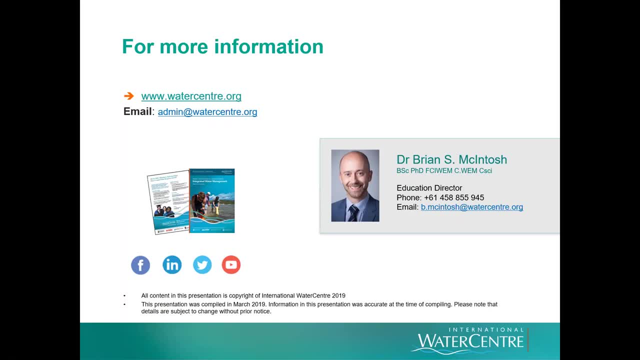 And that's therefore it's. it's at a smaller scale than than climate change, which really truly is a sort of global commons issue. When you get to water security, really, I suppose you're talking about hydrological basins. 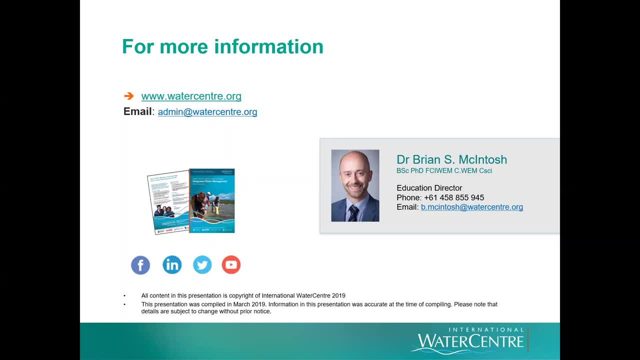 Of course it's. it's connected to to climate change, because climate change is is driving changes in the distribution and intensity of rainfall, which to some degree, is causing the water insecurity problems. So we need to make sure that we are. 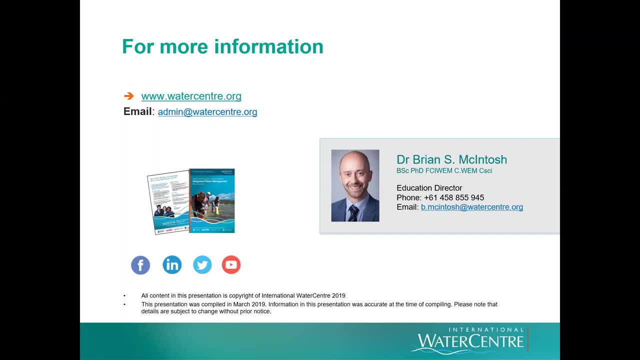 that we're we're thinking of. we're thinking and acting locally within the river basin, but also appreciating that some of the the influences on the river basin are are global. We also need to, I suppose to, to think and 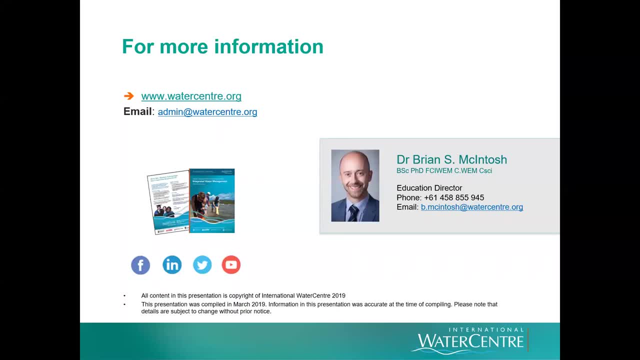 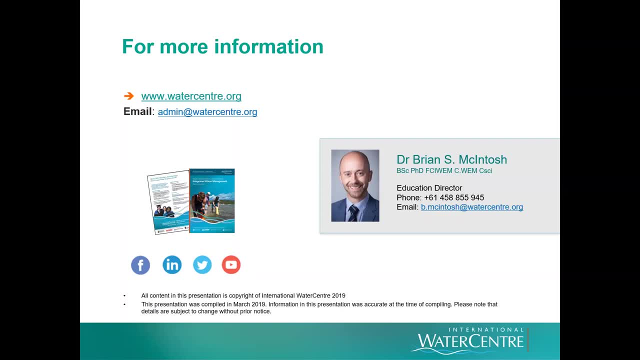 the direct flows and quantities of water in a river basin, You know, is there enough to to satisfy whatever the local demands are. It might be a mix of agriculture and urban and maybe an industry, But you've also, I suppose it's. 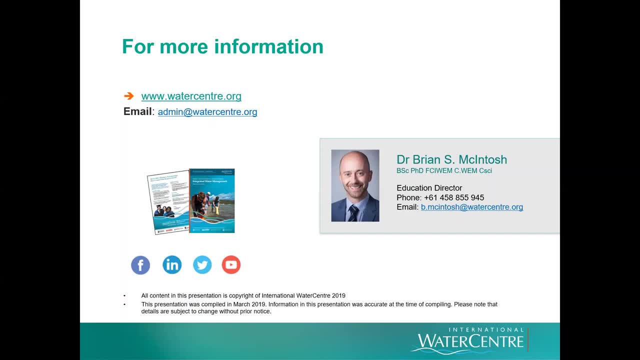 we're probably thinking about: well, where, where does, where else does the water come from? You know at king's college in in london a chap who's created the virtual water concept. he he always talks of big water and little water, and big water is basically agriculture and little water is. 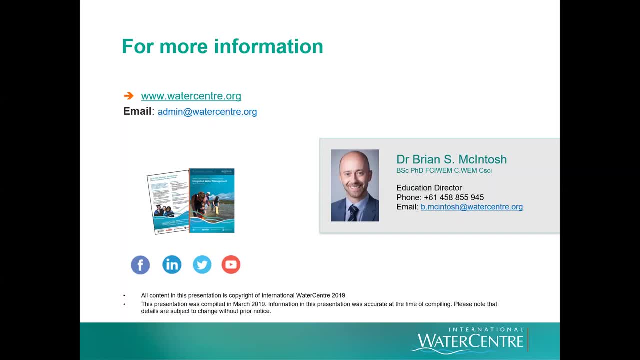 everything else from a human perspective. um, we know that in our agricultural produce we've got huge embedded water footprints, um, and so when we're talking about water security, uh, we've, i suppose we're going to be partly trying to trying to ensure that we are collectively at a local scale. 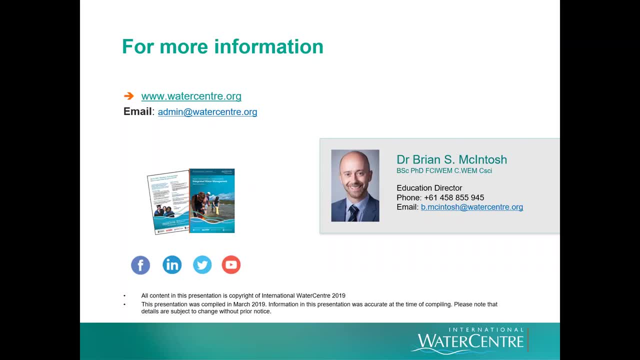 aware of where the problems might lie, and the problems might lie in terms of an, an, uh, an excessive dependence on imported foodstuffs and therefore an excessive dependence on uh, imported virtual water. um, you know, if, if water becomes scarce where, wherever your food comes from, then 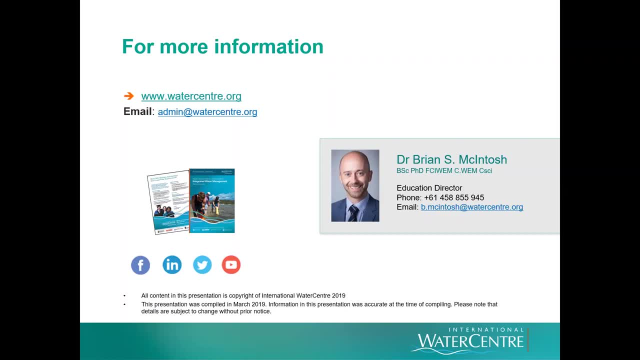 that that foods, uh, that food supply is either at risk of going up in price or or or of um of reducing in in quantity. so we, i think we've got to work collectively to um to become, to get. i suppose part of it's about awareness, you know it's the 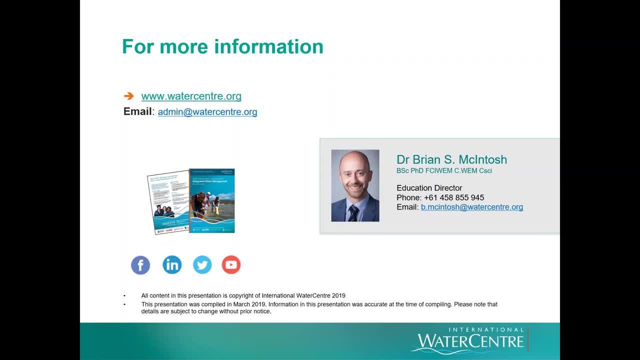 first process, first step in any process of changes is about, about awareness, and then, of course, you've got to start, then, uh, i suppose, outlining a, a vision of, of a collaboratively developing, and outlining a vision of: well, okay, so what do we do? where do we go? and then there's a process of 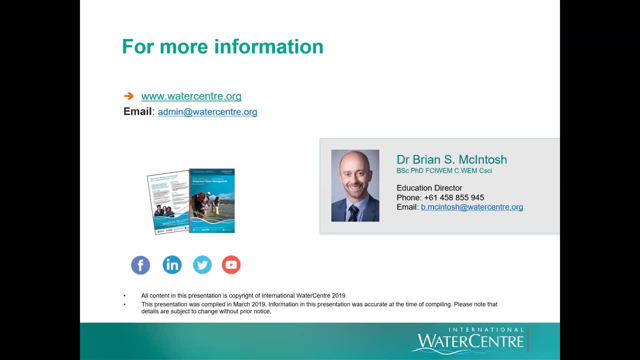 um, um, aligning uh resources and motivation and commitment to heading in the direction of of that vision. that's where we you start to need to to bring potentially in uh uh political will. um, and that's partly about the public, but it might be about politicians, or it might be about 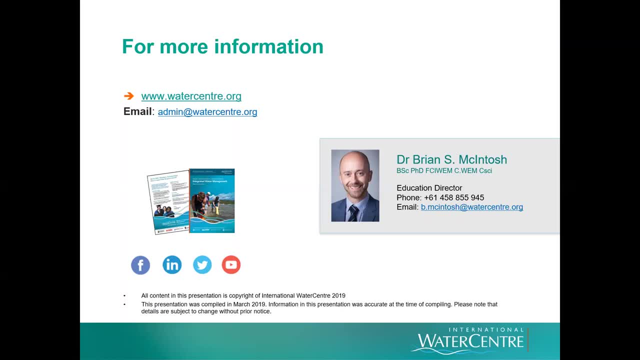 bringing on board senior managers from, um, from from whatever organizations are working locally, uh, with respect to water security. yeah, so that's that's a long, a long answer. no, that's fine. i mean, it was a difficult question. there's none, not just one resolution on anything. what we do, um, and i would like to build on it, but we have 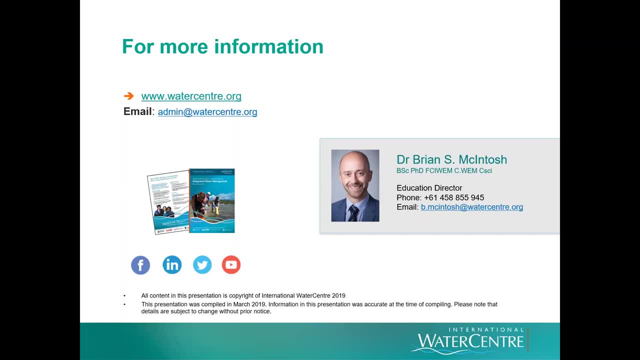 two questions in the chat, um, so, uh, one from edward is: does iwm have a water quality modeling? uh, yes, yes, sure, absolutely so. if you, um, if you don't, well, if water quality is an? uh an issue, then um the reason why the edward study was so critical. um the reason why the edward study was so critical. 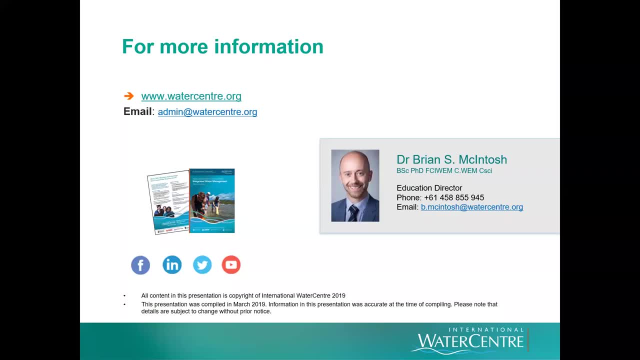 was that um the ability of the government to um to uh on a water quality level? um, i understand that there are uh very high levels of water quality uh in the area of the water management um, but i think uh the the work that has been done in that area and the effort that's been made. 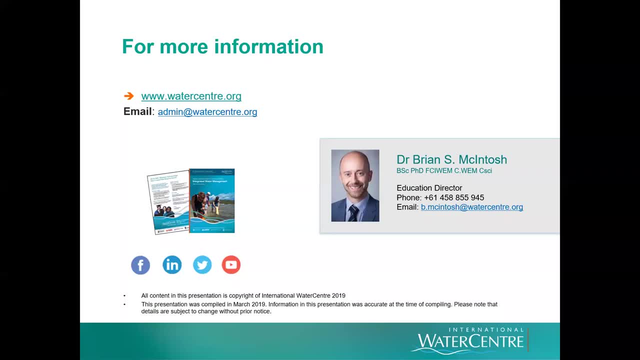 in terms of uh, in terms of um uh, navigating, uh, uh, how how the water is um, uh, uh, what, how is the how the how the water is used, um and and the iowa area on the flora and fauna, just to kind of Barrier Reef Lagoon. The Barrier Reef Lagoon is basically the bit of water between the coast and 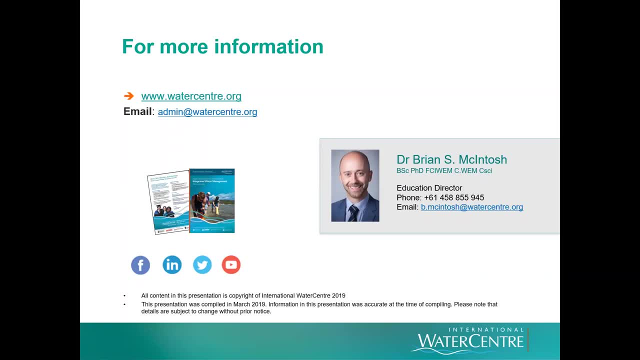 where the Barrier Reef properly starts. There's a whole range of catchments, some fairly major rivers, some smaller rivers. Some of those catchments are natural. you know they've not been cleared for agriculture but there's a reasonable amount of land there which has been. 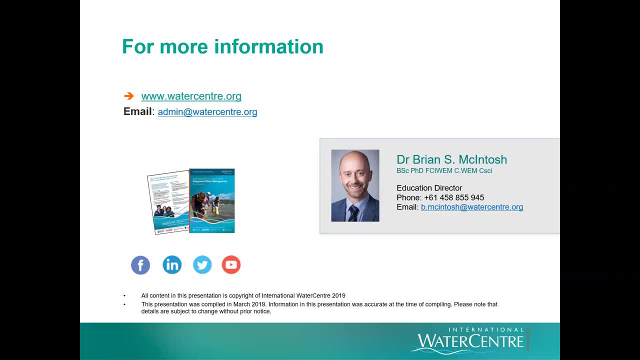 cleared for agriculture. So what the Queensland Government has done is set up- I'll call it- a system whereby there is water quality monitoring, which is feeding into a fairly highly developed set of models for each of the catchments, which are then translated into action by a set of NRM. 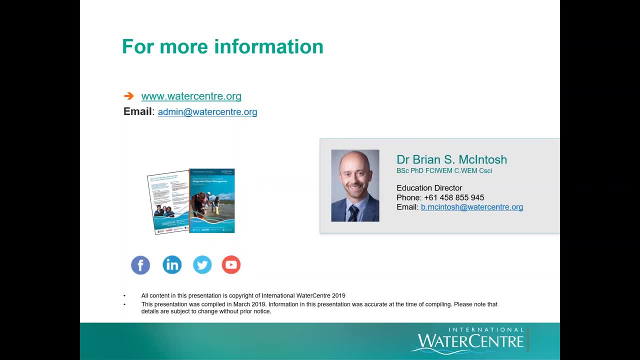 Natural Resource Management. So Queensland Government does the monitoring and it does the modelling, and then it's translated into management action. You know farmers practising differently in terms of fertiliser application or cropping patterns. It's translated into action and the constraints on action are: 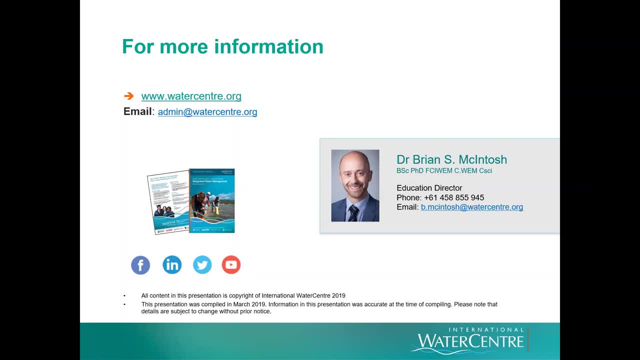 fed back into the Queensland Government by these things called NRM groups- Natural Resource Management groups- which work directly then with farmers and with agriculture. And now we're back to the process of monitoring and monitoring not just for getting them into middle ground but for the people that are coming in and into the nearing returning areas. 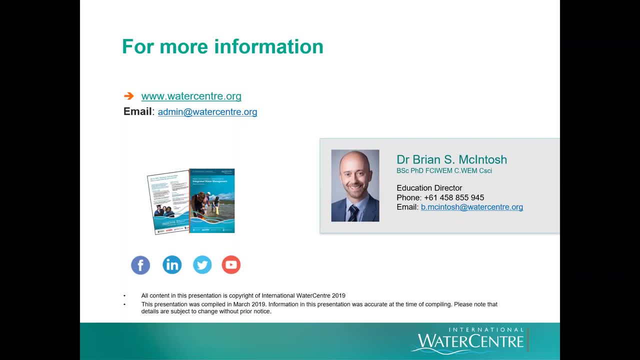 And the digitisation of these. you know the diversity of those geological fields. In fact, from the previous slides I've written about when I was doing my review and I found out that the nitrogen load is also very low. but it does. it does cross the grid And that's why we're doing the monitoring and the modeling. 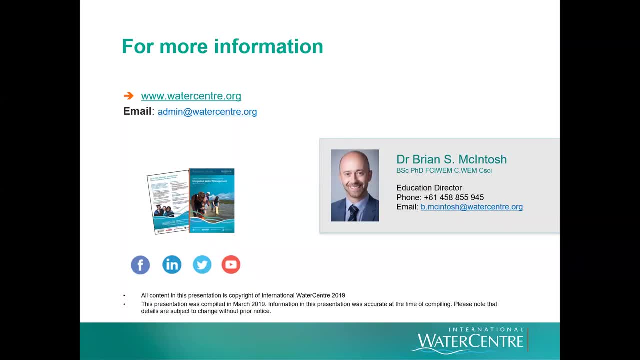 If that's the case, then the best place to make an impact on reducing nitrogen runoff is in in the water quality modelling is in those three fields, and so work directly with the farmer or farmers that use those three fields for production. So yes, so look, I think. 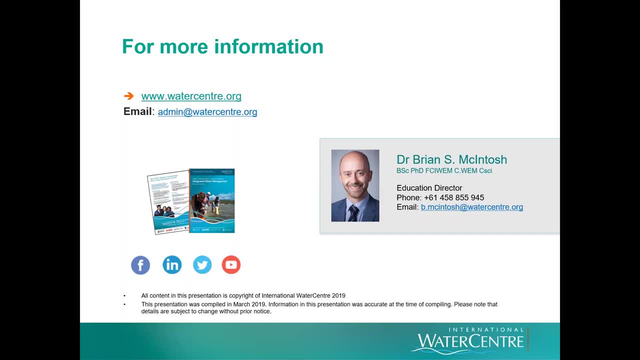 where you've got complex, large, potentially large-scale processes like water quality change and the relationships between land and runoff and river health, and that modeling is an essential tool. you've got to make sure, though, that it's. I suppose there's two ends. one is the 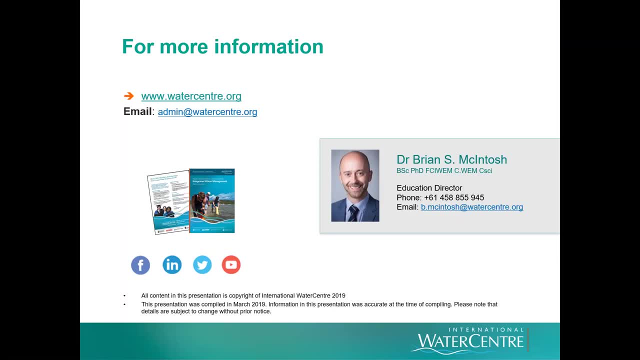 input, end or input side. if you don't have good monitoring, good data to go into models, there's the phrase: giggle garbage in, garbage out, you're gonna have nonsense coming out. but you've also got to make sure that you've got good trust. 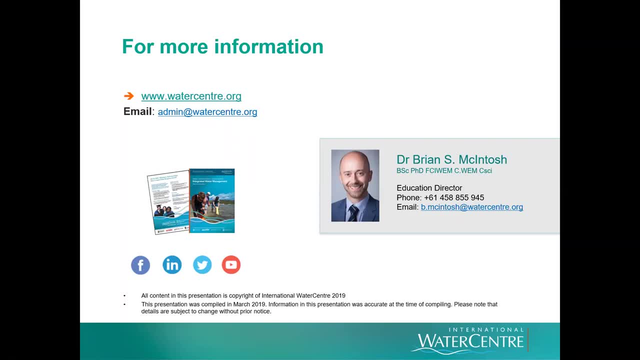 you know, it's no good having a bunch of modelers sat in a room creating forecasts and then farmers go: don't trust the science, don't trust it, Don't trust them. So you know, actually to make modeling more accepted there's got to be engagement, whether it's participatory model or modeling or 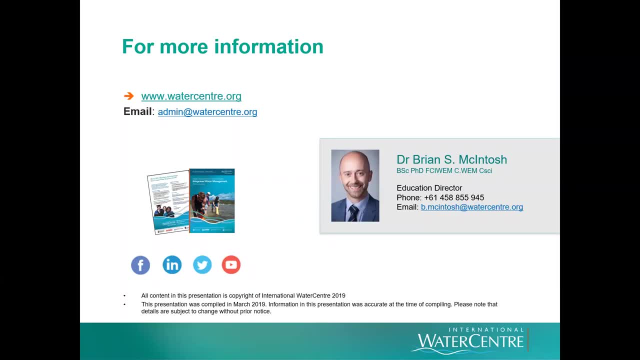 whether it's something a bit less than that, I guess, depends on the context. So look, yes, I would say IWM does include- can include- water quality modeling. if that's relevant to the situation, Great. thank you for the question and for the answer. I think I know for personally: modeling without measuring doesn't work. 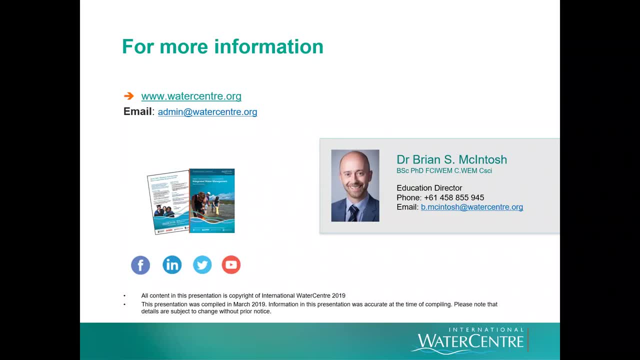 models are only as good as the data you produce. But the next question from Camilla. so what do you think is the biggest challenge for use IWM in projects? What do we challenge when we speak about? Yeah, so it's probably. it's probably at the design and scoping. 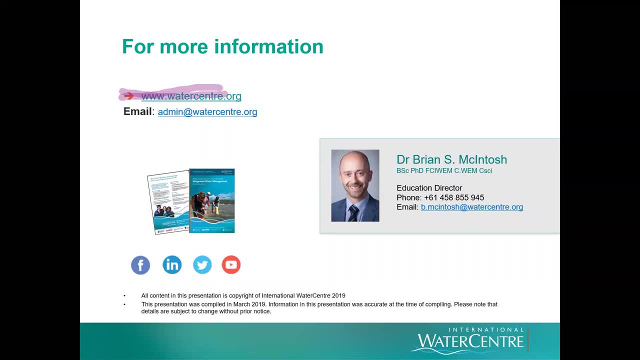 stage, Once a water management project has been scoped and designed and planned and budgeted and money's been granted, it's kind of difficult to shift it. It's sort of locked in to some degree. So I think perhaps the biggest challenge is in taking an IWM approach to the 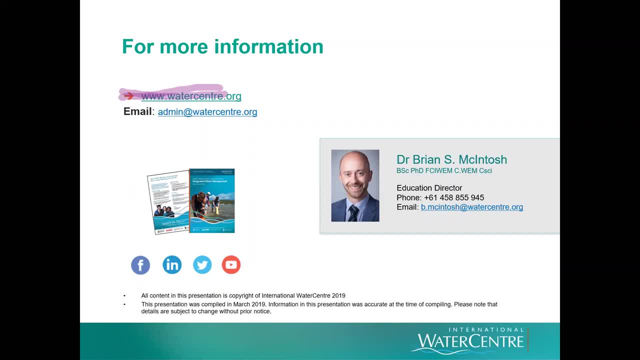 formulation, to the design, to the scoping of projects, so that there's time at the beginning to figure out what you don't know you don't know and incorporate, incorporate that then into the project design There is, there are some challenges that we've got, I think collectively, in terms of the way that we 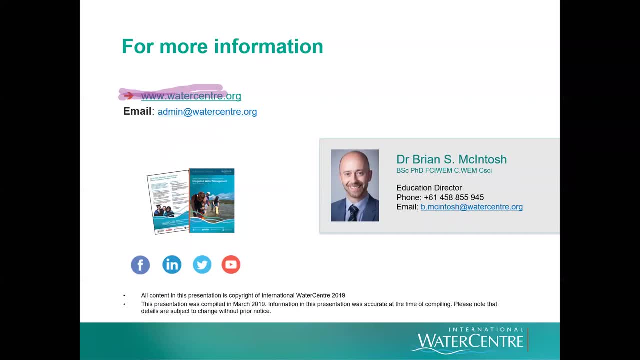 structured and deliver work. The projectification of work. If you look at how I suppose even just that, that reef catchment work that I was talking about. sure, we've got some government custodians and owners of the models, but the the point of engagement with farmers and stakeholders on the ground, 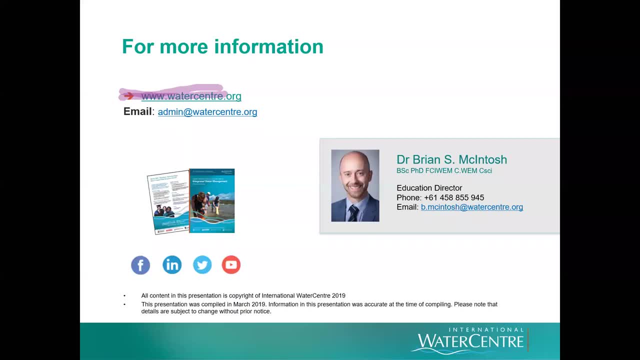 for both understanding their concerns and influencing them to change their practice. you know that that's funded in projects and programs, which means the NRM groups are. they find it really difficult to to to maintain their knowledge over time because their funding isn't long-term or 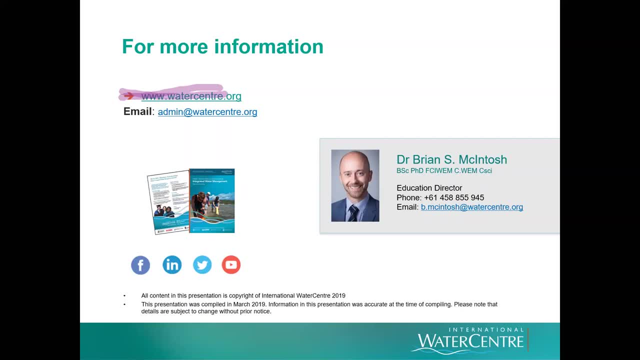 guaranteed. so we end up with institutionalization of knowledge problems because we chop the world up into projects. We also problem owners in the sense perhaps governments commission consulting firms to to do bits of work for them. the consulting firms do do them as projects and then move on, and so the again it's about institutionalization of. 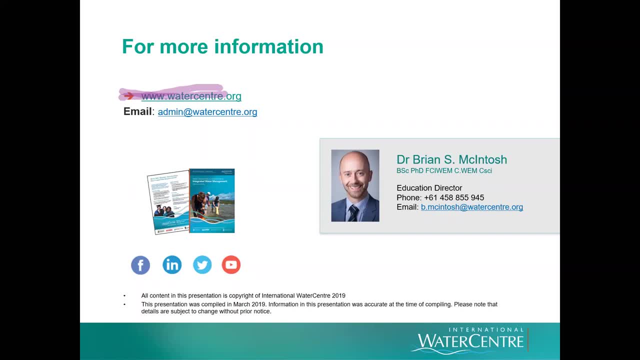 knowledge and and building up over time a proper understanding of the whole situation. if the way that we organize work work means that sometimes it's not clear really where the knowledge is being built up at an organizational and institutional scale and the knowledge exists, a project scale, but which is all sorts of bits. so I I think that's two. 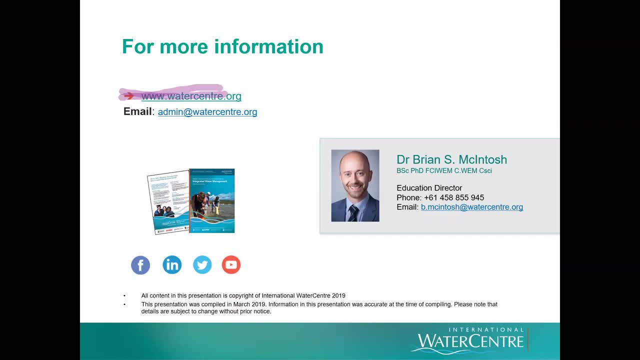 two big challenges to to IWRM. One is is at the individual project level and the second is that the is that the sort of, I guess, a larger sort of- how do we build up institutionalized systems, knowledge? So that's all partly a problem of projectification, you know, chopping up work into projects. but 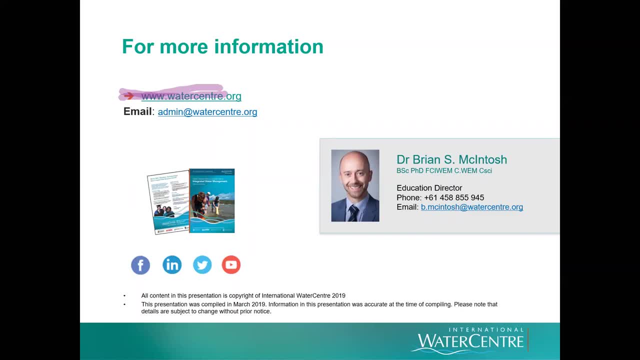 it's partly also a problem of of governance and roles and responsibilities- is difficult inside an organization to do something that's not strictly within the remit of that organization, and water utilities, for example, find this difficult to do. most water utilities are mandated by by by law to provide water and to dispose of and treat wastewater. they they're not really. 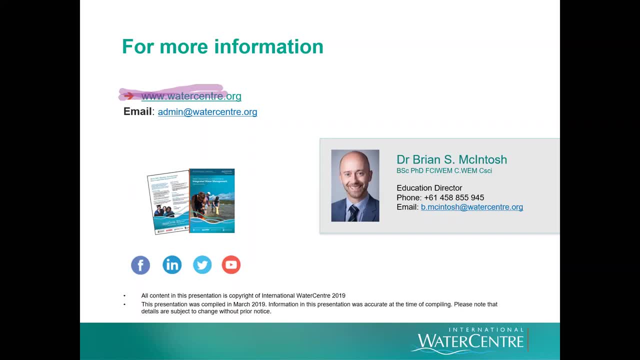 mandated by the law to produce biosolids, compost products or or to produce energy, and and so it's. it's difficult for people working in those organizations to to really take a whole of systems point approach and and and recover materials or generate energy, because it's. 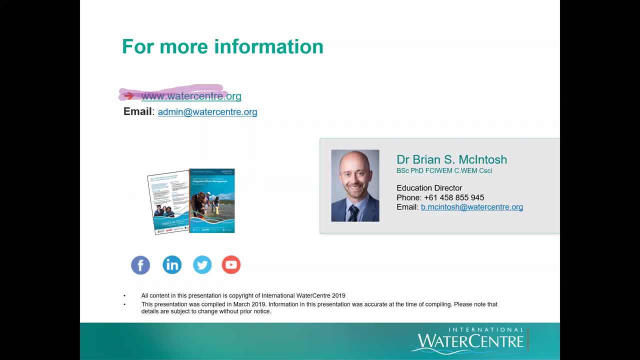 just not inside the mandate of the organization. and if your senior management are of the view that the organization should do what it's set up to do, then doing something that is not set up explicitly to do but which is not prevented but it's, it's that's. that's a hard thing to get to get moving. 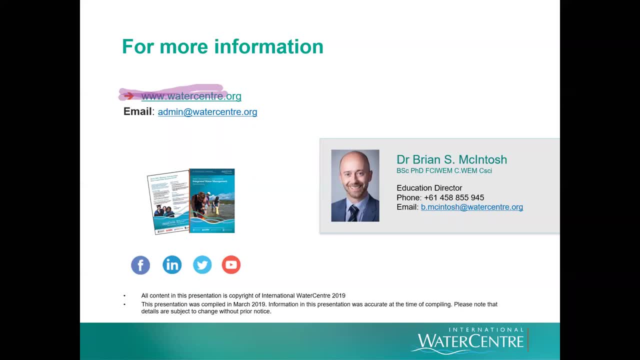 Okay, great, thank you. so if no one else has a question, I maybe have just a last quick question to finish. maybe this, and it's probably one of the hardest, but maybe the shortest answer you get out of it- what do you think, professionally, is the hardest to communicate with? this is the public. 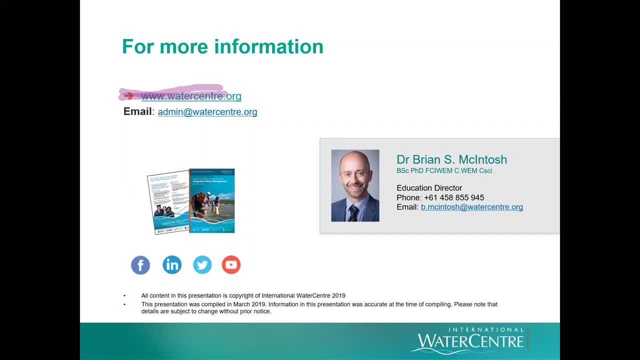 other communities or actually industry politicians? hmm, that's a good question. I have a suspicion that the way that politicians and media interact, they've there's a sort of a dysfunctional relationship, I think, which has emerged over the last decade to 20 years perhaps, between media and politicians. 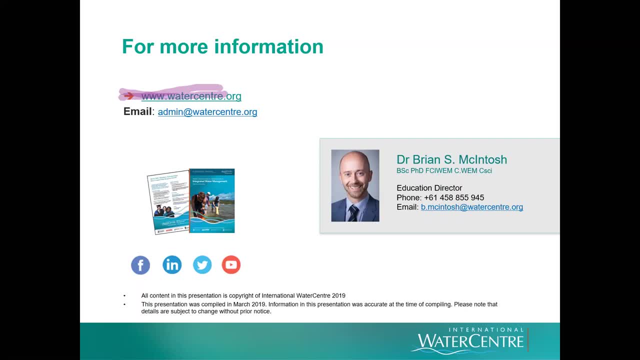 you know, there's 24-hour news media, which makes politicians- I think that's partly what makes politicians behave as they do and speak in the sort of funny no-speak that they they use- um, so cutting through to politicians and and working with politicians when they're in this, quite kind. 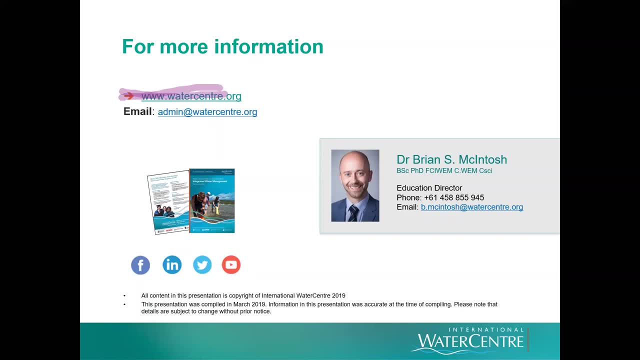 of dysfunctional. they need to show results, and uh announceables all the time, uh to because of the 24-hour news sort of cycle. that's, that's a significant challenge, Um, but in a sense it's the same as it's. it's the same challenge as you you'll get with communicating. 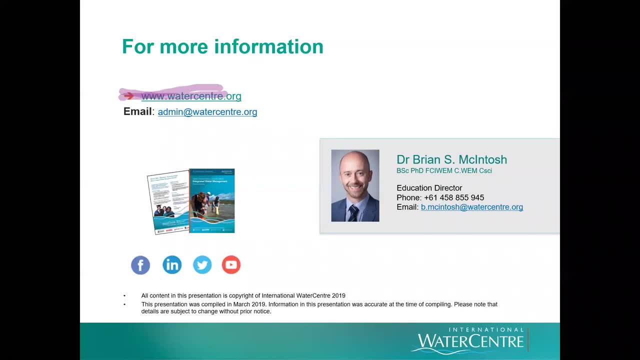 with any stakeholder. it's all about trust. people will will listen to you if they trust you. so, whether you're talking with communities, or whether you're talking with politicians or senior managers, you've got to spend some time to to generate trust. um, uh, and so that people unders, I guess, view. 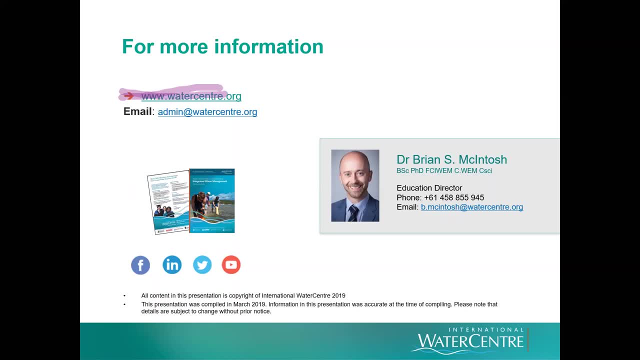 whatever you're saying positively rather thanум, you know, in a more concrete way, negatively, um, and trust takes time to to develop, um, it's not something that can develop instantly, and it is something that can be destroyed very quickly though. so you know, enabling what i suppose. 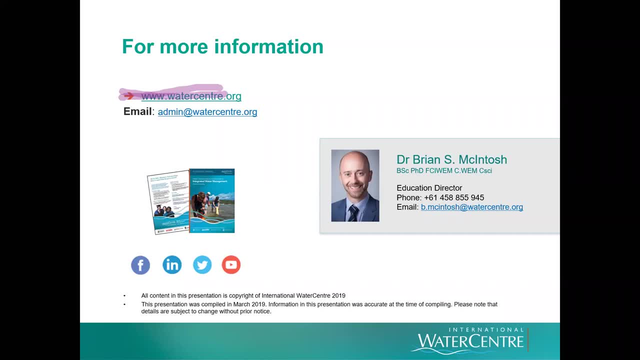 the answer. perhaps politicians are difficult to talk to, but to some degree the problem is, it's just all about trust. you've got to make sure that you invest time, um, in in generating that trust. okay, never thought about this, about the trust, but yeah, you're probably right about that. 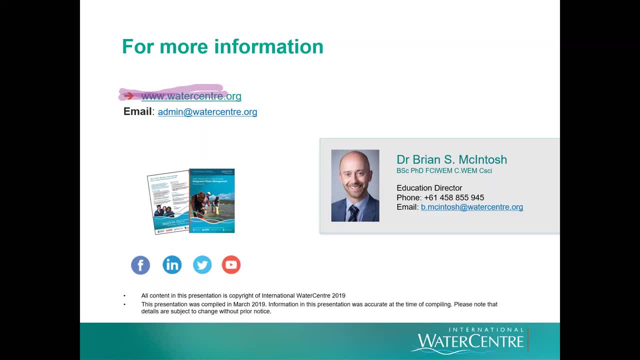 um, it's the, it's the, the oil of social interaction. nothing happens without trust. i know, um, it's just. i think we're just producing so much data to um produce knowledge, but uh, we don't put too much effort in it to build the trust. that's probably. but yeah, um, it's was really. 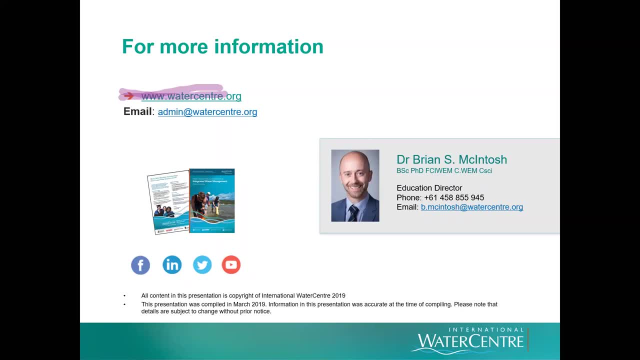 really interesting talk. thank you so much, brian, for giving this webinar and this presentation, and no, that was a pleasure. i i hope it. you delivered something of use to to to everyone. uh, iwirm is such a huge topic. you could have all come with extremely diverse expectations of what was going to happen. so hopefully it uh, hopefully. 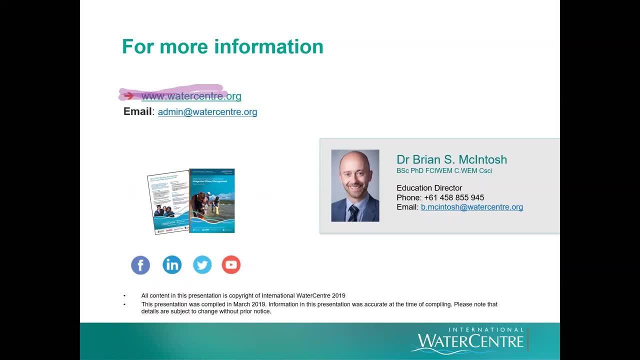 it delivered. uh, something of value to everyone. for me for sure, because i'm pretty new in this topic, um, and thank you for everyone who participated today and for asking questions, and i hope we can stay in contact and build something together with the water use network- really happy.